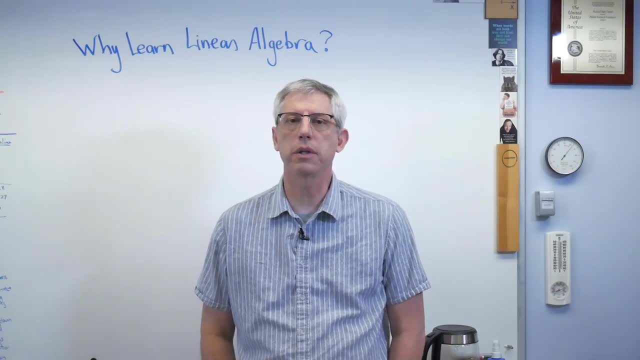 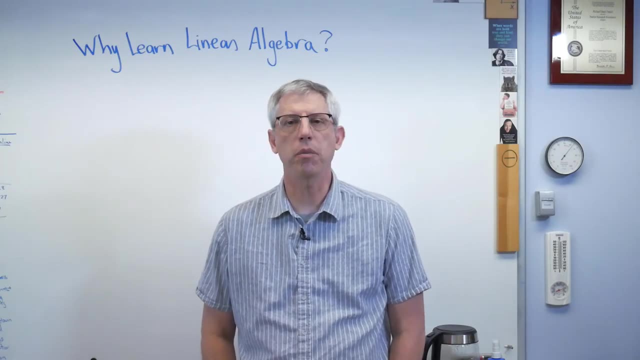 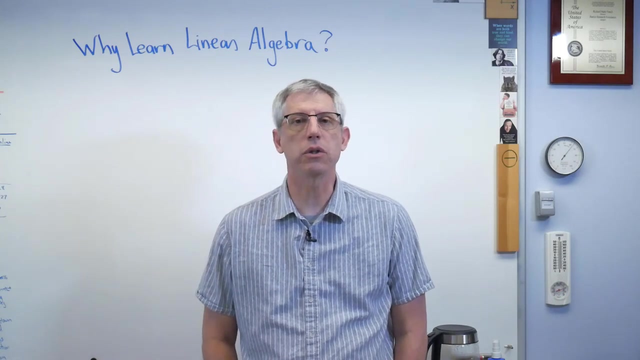 So linear algebra is a class that you'll take if you're in one of the sciences or in engineering, maybe some other fields, and it means different things to different people, And I think part of the problem in learning linear algebra is it often means different things to the professors than it does to the students. 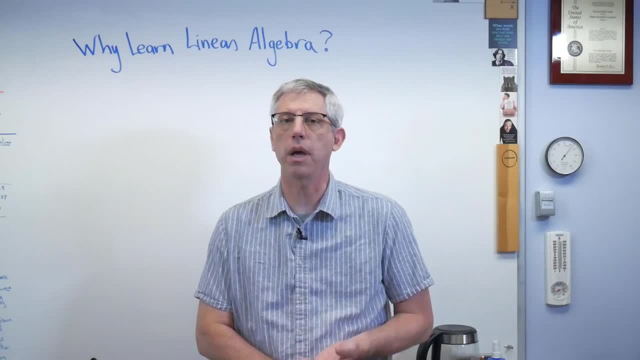 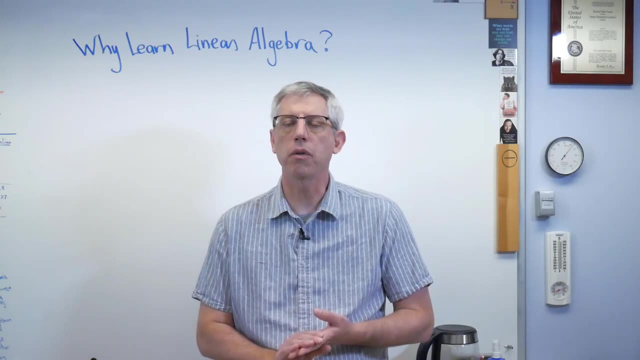 And so what I want to do is I want to go over a simple example of linear algebra, so we make sure we're all talking about the same thing, and then I'll go over a little about the motivations for different people to either teach it or to learn it. 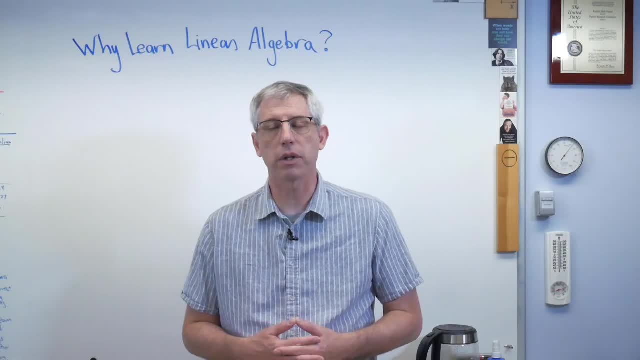 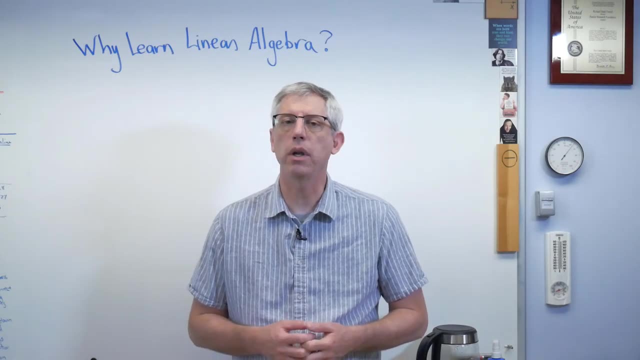 Alright, so let's get started. Linear algebra is just what it sounds like: It's working with systems of linear equations. What's a linear equation? A linear equation is one where all the variables x, y, z, whatever you want to call them. 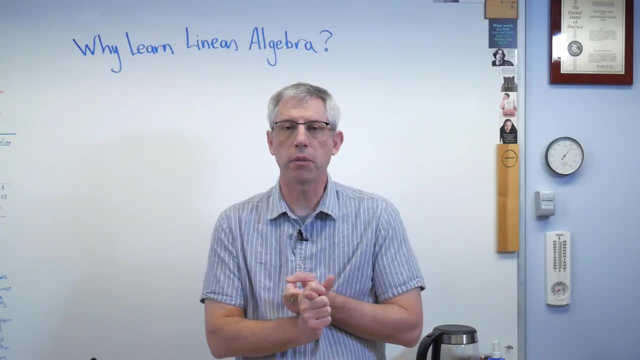 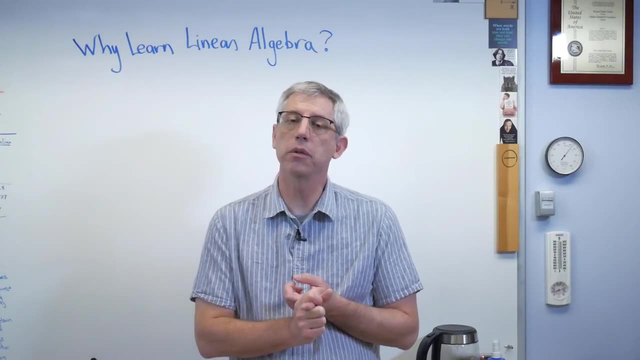 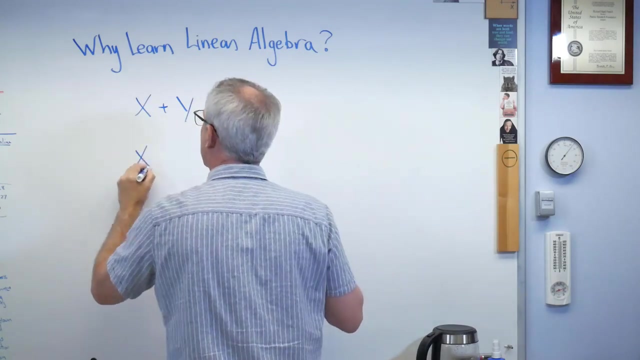 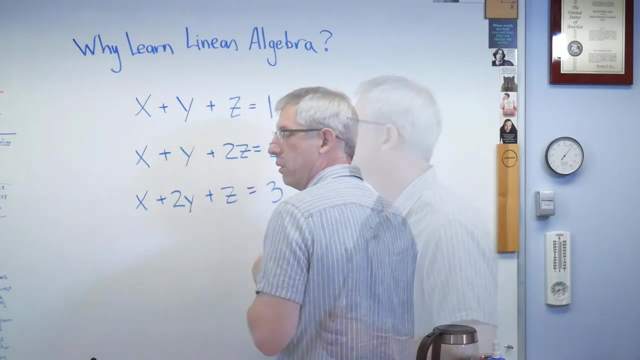 Are all to the power of one, and none of them are squared and also none of them are multiplied by each other. So here's a real, real, simple example of a system of three linear equations. Alright, so here's a system of three equations and three systems. 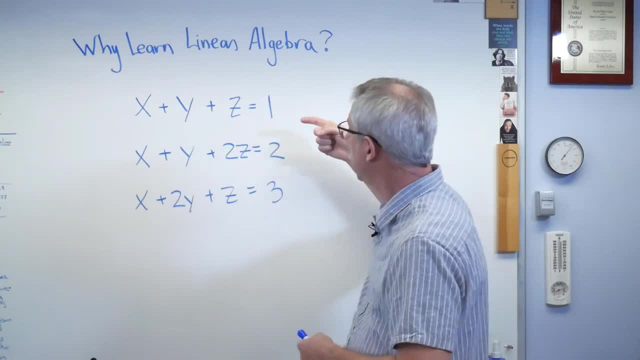 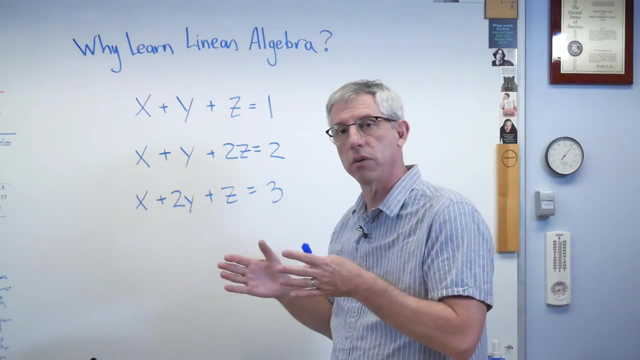 There are three unknowns. The unknowns are x, y and z. Those are the variables, And there's equation one, equation two and equation three. So fundamental theorem of algebra gang: If you have three unknowns, you can need three equations to solve for them. So here they are. 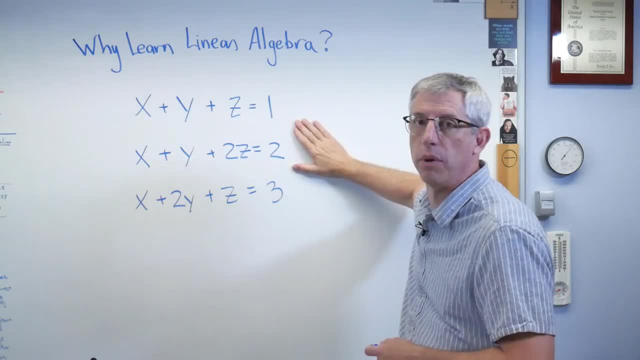 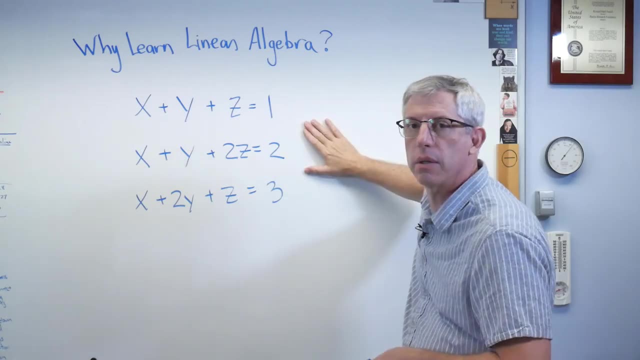 Now what does this mean? Well, inherently nothing. It's just a system of three equations. Now it becomes interesting. You want to solve it when you have some reason to solve it. Maybe this describes something interesting about the world around us. 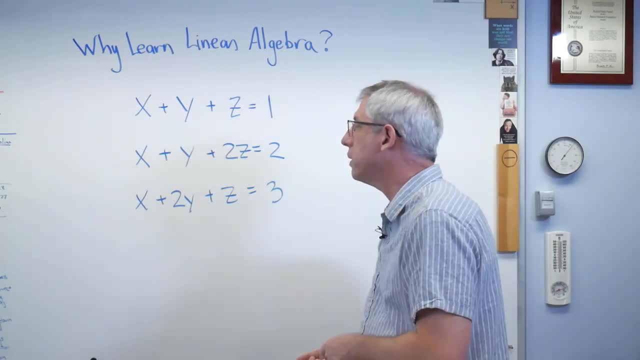 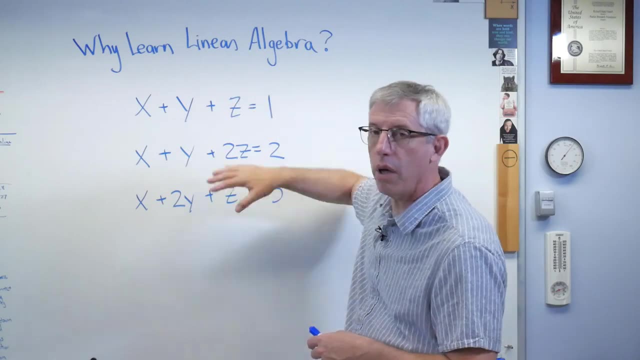 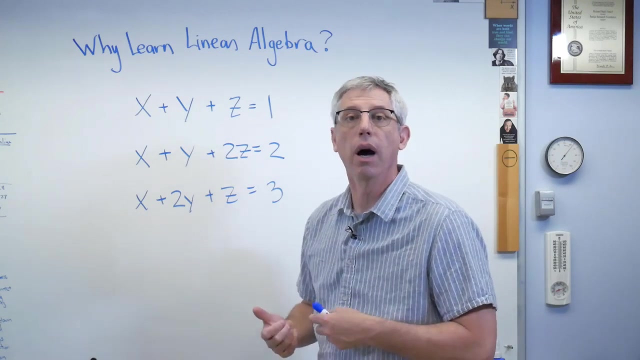 Maybe it describes some engineering product or process, or some financial model or something. There's some reason that we have to write these equations down, And solving these equations will give us a result that is useful to us. That's why you want to do this, Unless you're a mathematician. 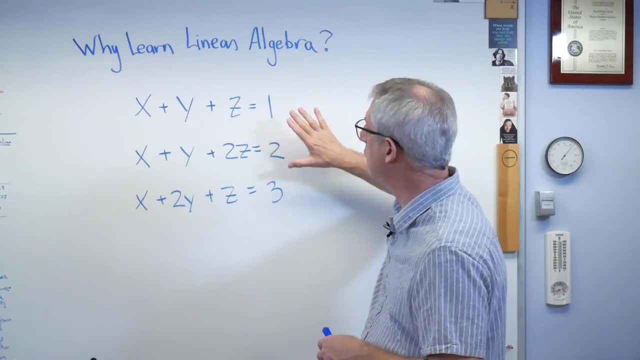 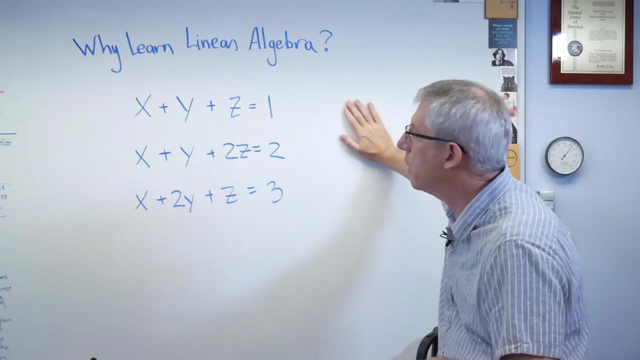 And then the goal is to explore mathematics, Then the act of exploring this is the reason for doing it, And that's just as valid. Okay, How are you going to solve this? Well, let's see, There's a bunch of ways to do it. 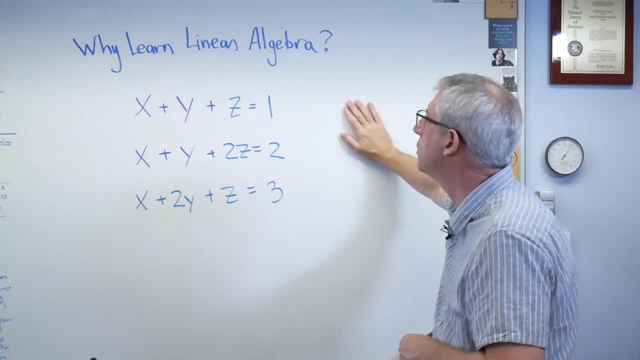 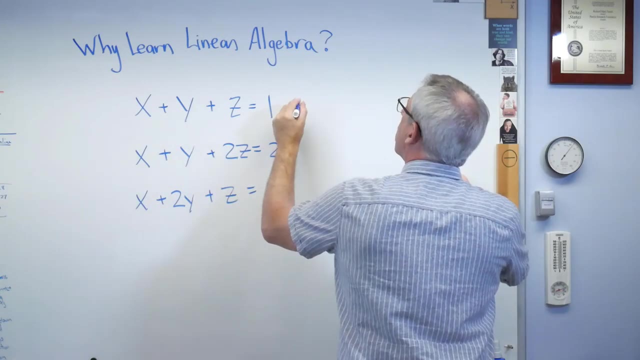 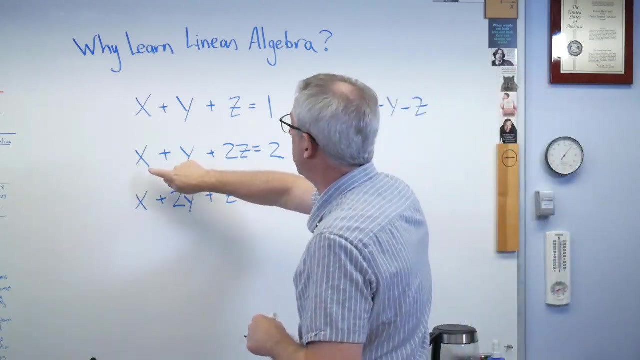 The easiest, the most straightforward way probably is called substitution. Well, if I wrote x equals one minus y minus z, I'm going to put here, I'll just do that right now. Okay, so if x equals one minus y minus z, every place I see an x, I can replace it with that. 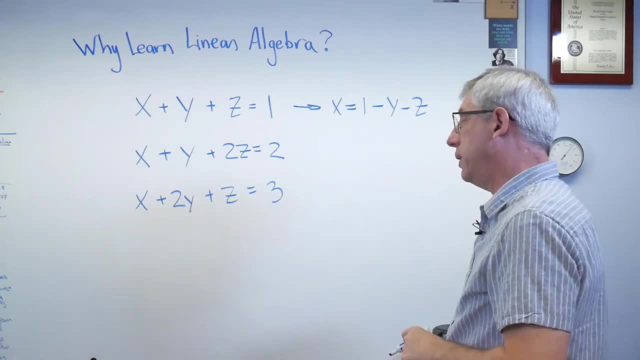 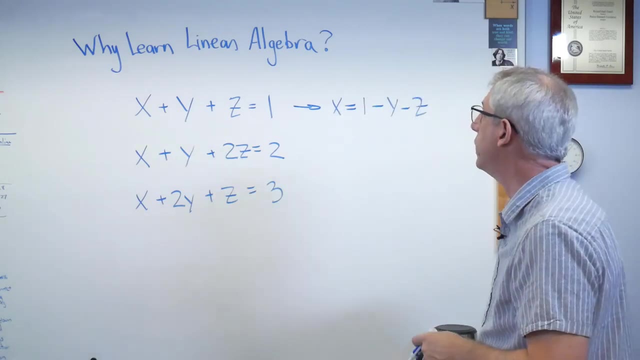 Alright, That gets me down to. let's see two variables I don't know, And then I can do the same again with y and eventually solve for z. It's called substitution And that absolutely works. There's nothing wrong with doing it. 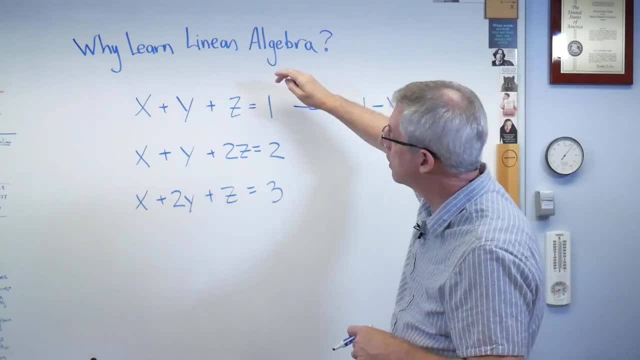 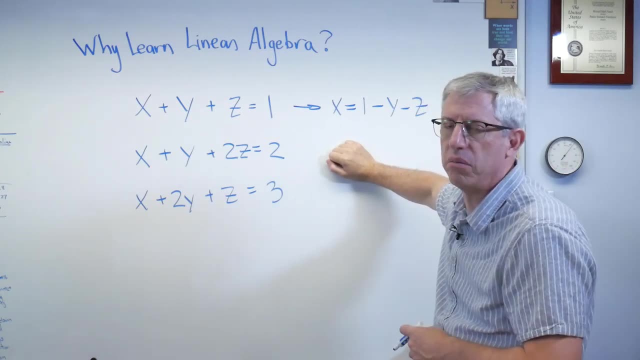 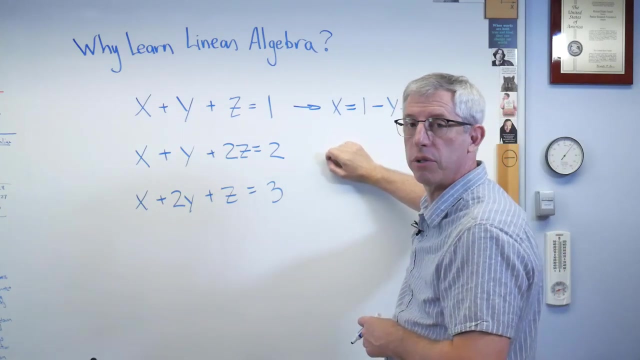 The problem is it gets awkward as the number of these equations gets large. This is three. What's a large number of equations? A million, Ten million. That happens absolutely all the time. There are engineering models, structural models, where a million equations and a million unknowns. 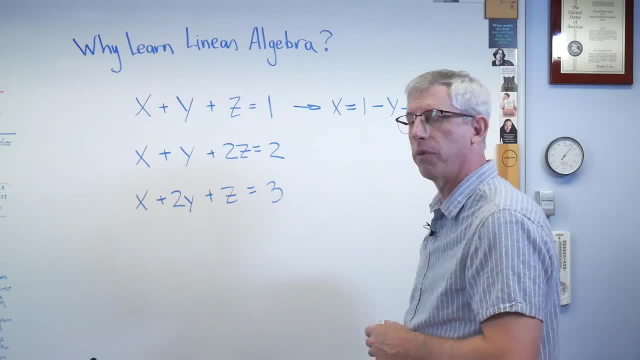 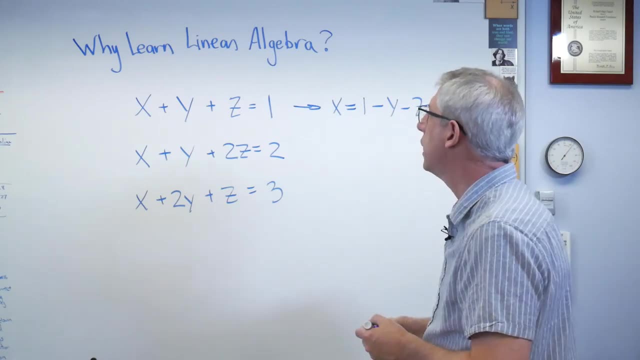 really isn't that big a deal. That used to be stuff for supercomputers, now it's stuff for desktop PCs. So substitution is not going to work with a million variables. There's got to be some other way to do this, and there is. 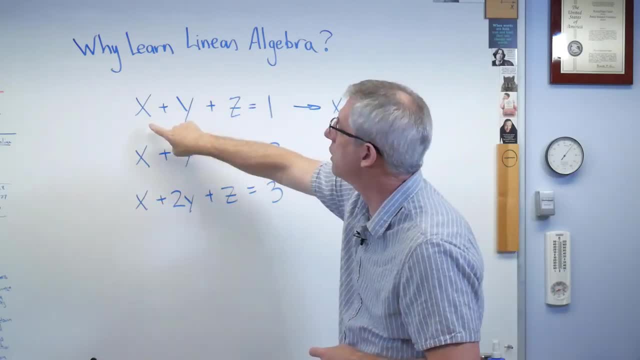 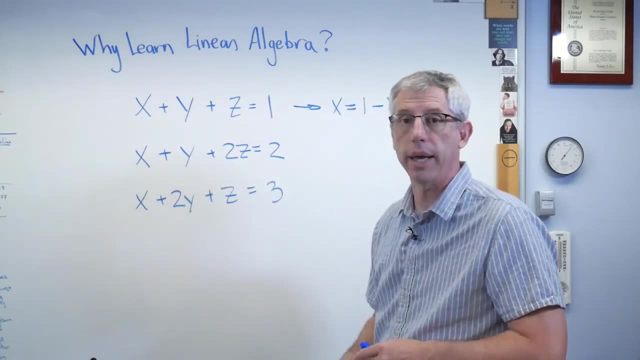 That's linear algebra. Linear again means we've got linear equations: x, y and z. all of them are raised only to the first power and none of the variables are multiplied by each other. What this looks like in three space, if I drew pictures of this. 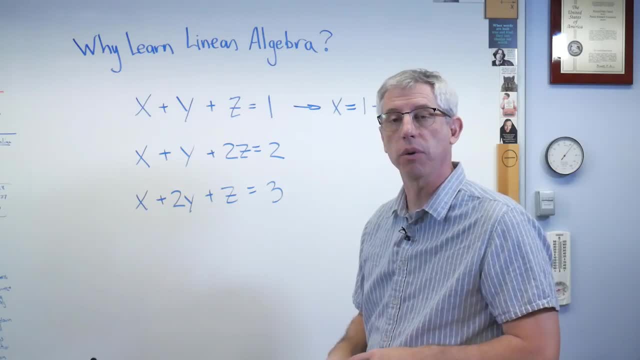 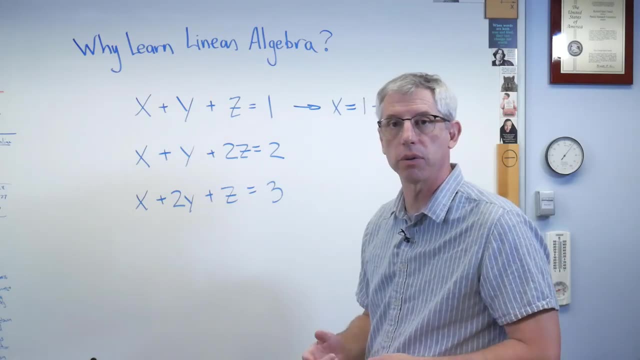 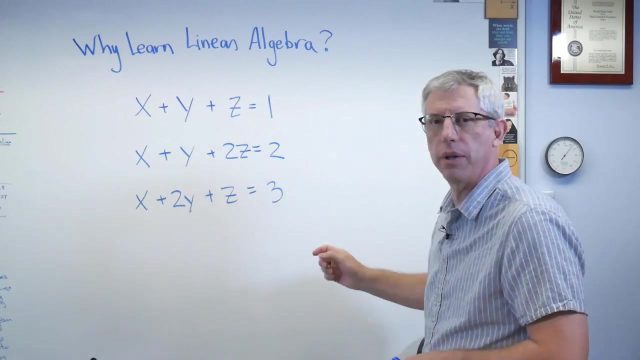 what I would have is three planes, Three flat surfaces that intersected at one point, The place where those planes intersect. that's the solution, That's what it looks like. What's another way to do this? Well, I need to think of a more general way. 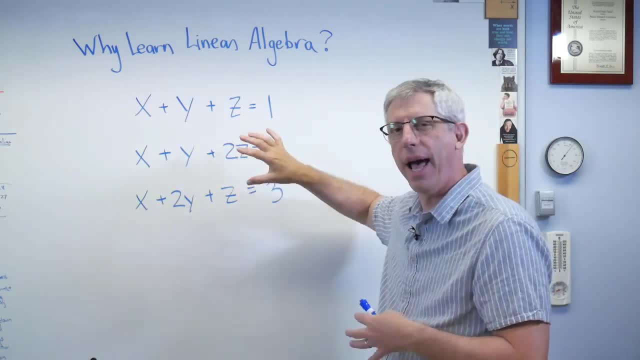 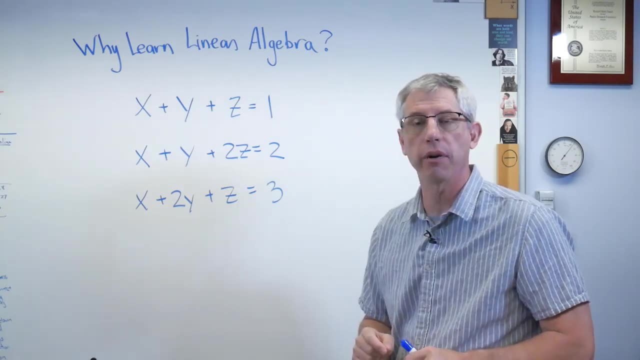 I need to abstract one level to go from this to something that acts like this but is easier to work with. That's where the mathematicians come in, and this is where some of the real value of linear algebra is. I can give names to all kinds of things in mathematics. 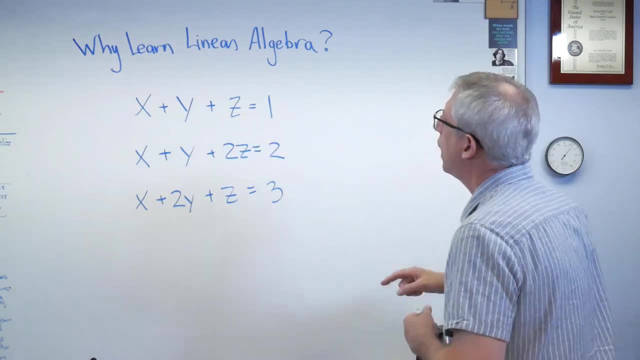 It doesn't have to be just variables. So here's what I'm going to do: I'm going to take this exact same set of equations and I'm going to write it slightly differently. I'm going to write it this way: 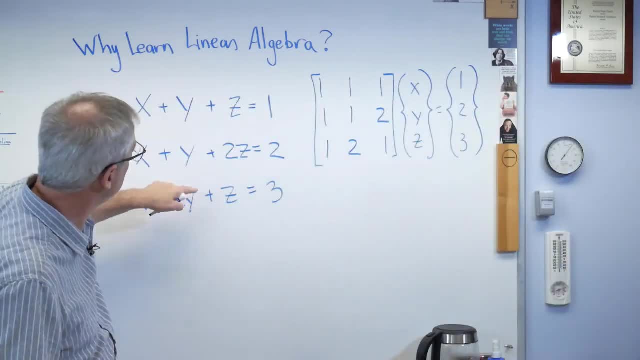 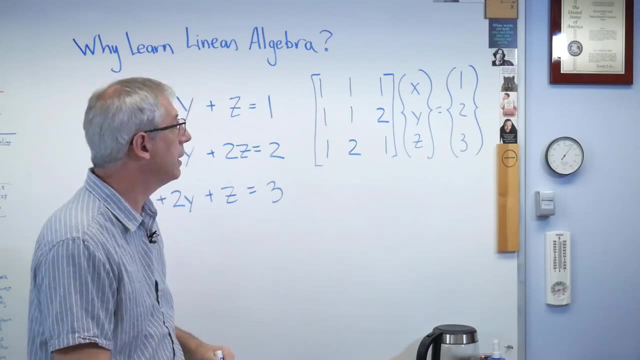 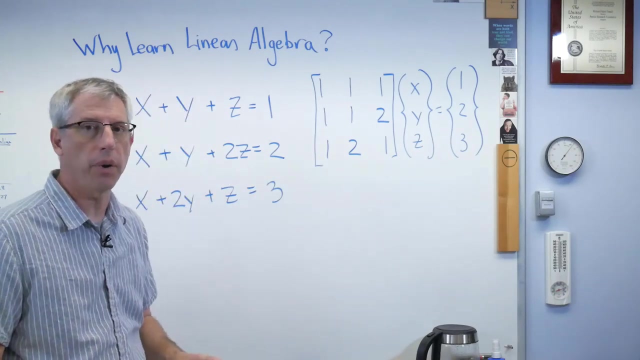 All right, All I've done is write down this exact same set of equations, but I've used a different notation. This is what the notation for linear algebra looks like. It means exactly the same thing as this. It's only notational at this point. 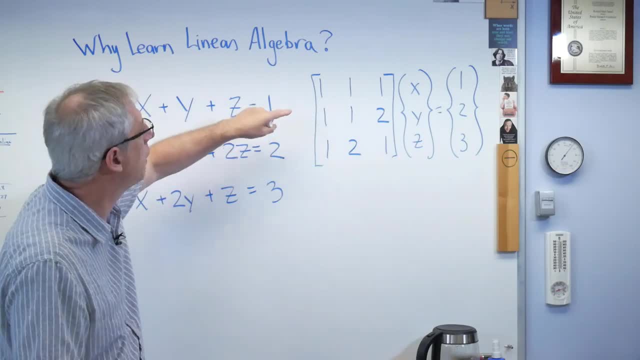 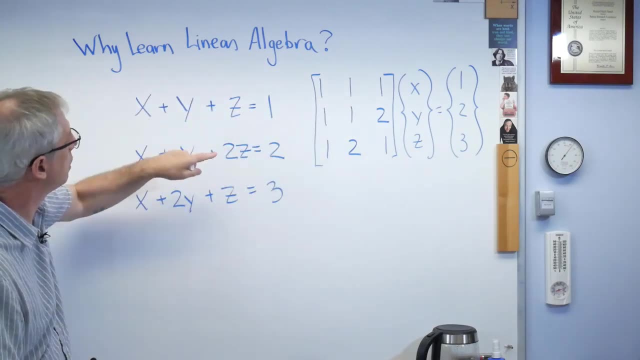 We'll get beyond the notation here in a minute. I just got an email, So what lives in this box? here those are the coefficients of these variables here. So one x, one y, one z equals one. Well, since it's one x, one y, one z, 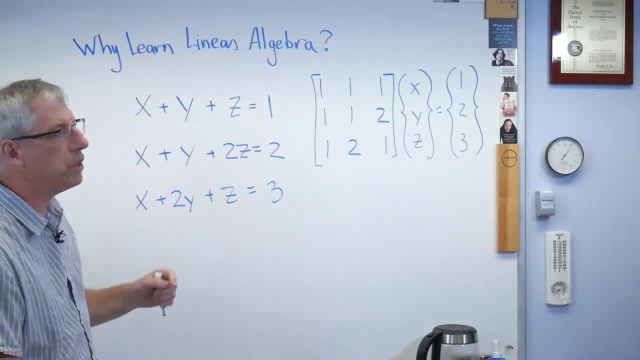 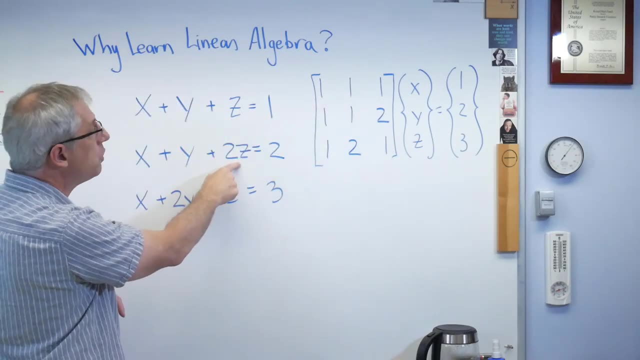 by convention. we leave the one off. You don't have to, but we do to keep things tidy. So there's one, one one. I have one x, one y and one z. I have one x, one y and I have two z's here. 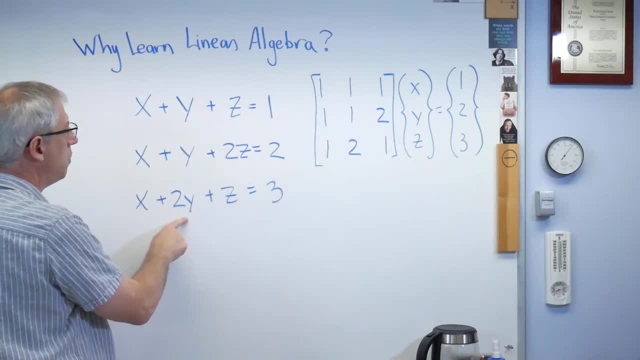 So there's one, one, two Here. I have an x, two y's and a z. So there's an x, two y's and a z. Now how do I know what the variables are called? 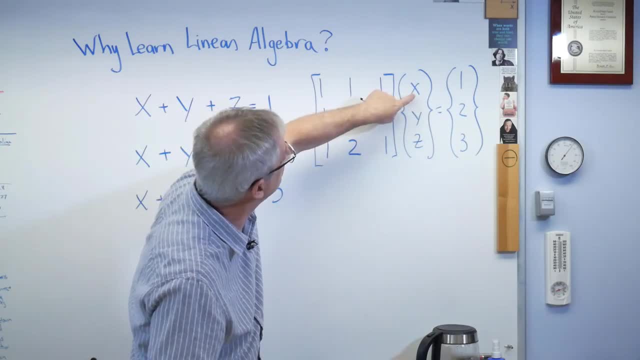 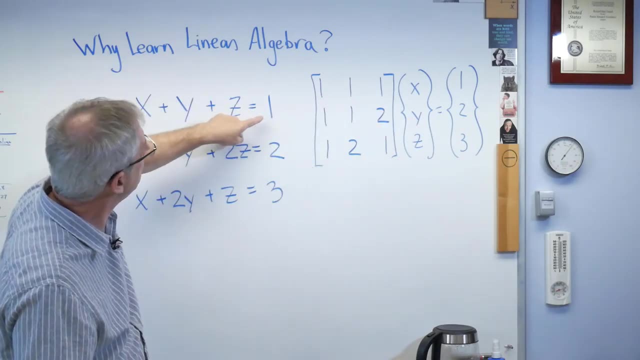 Well, that's what lives over here, this little column of numbers, x, y and z, column of letters, I should say So. there's the names of the variables, And on the other side of the equal sign, I have a one, a two and a three. 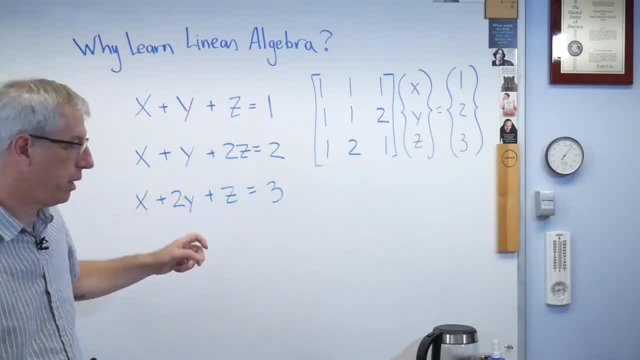 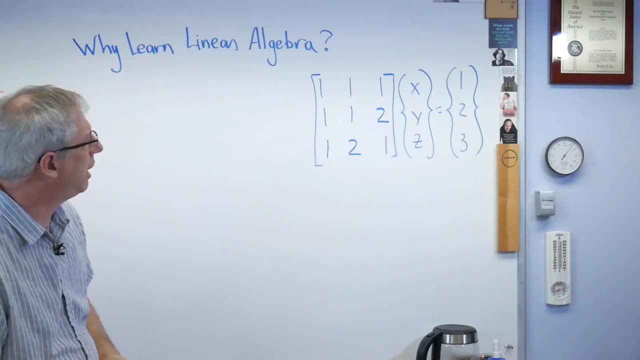 Well, there they are there. one, two, three. All right, I don't need this anymore. That's a little more general, but I'm not sure how, what to do with that. There's one more step we've got to go through. 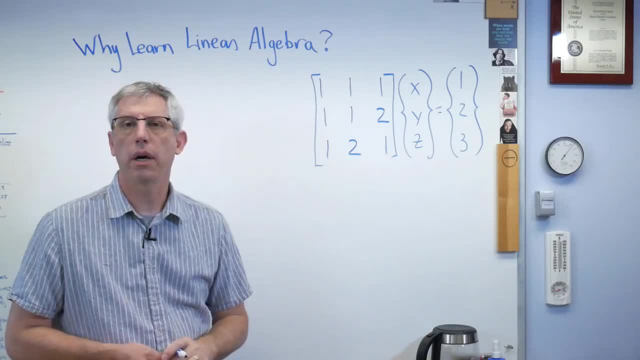 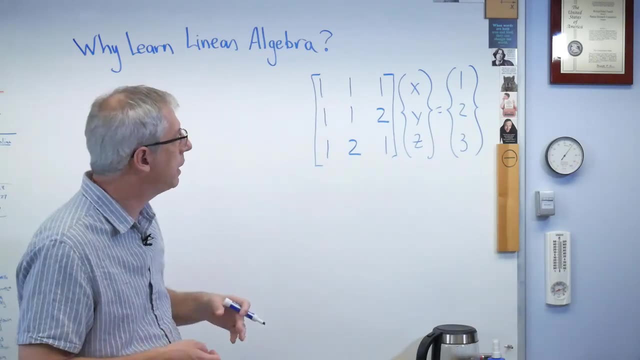 to make it general and go from just a notational convention to something that actually looks more like algebra. I'm going to name these. One of the things mathematics lets you do, and one of the things that makes it so, so powerful, is that I can take an entity. 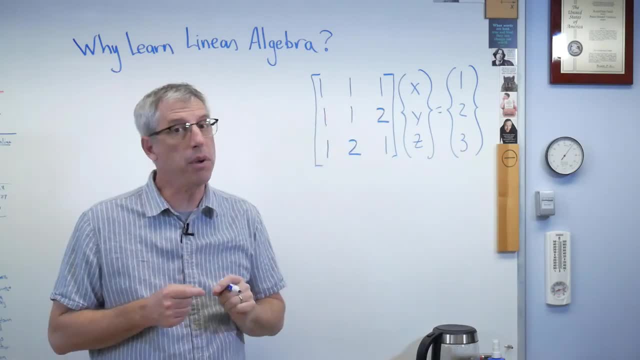 that may have a lot of content to it, and I can just give it a name and work with that name. So what I'm going to do here is I'm going to call this a and I'm going to put it in a little box there. 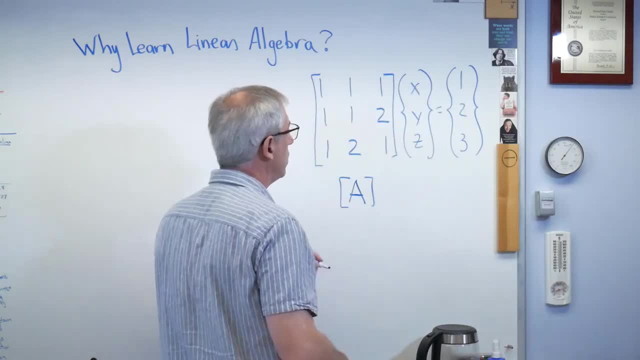 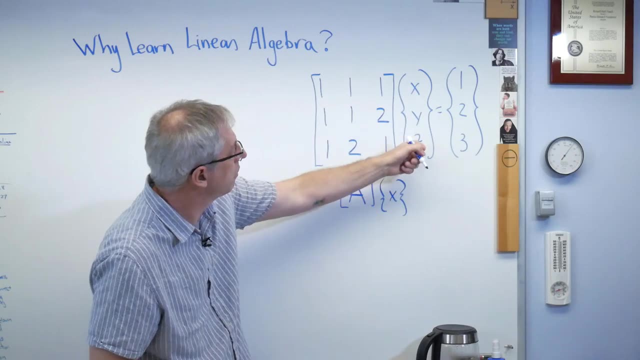 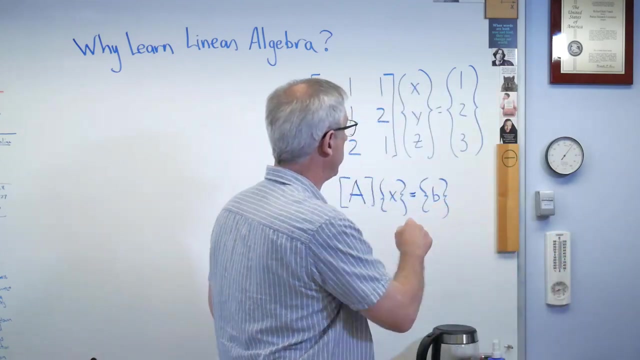 so we know that a is a box, just like this is. I'm going to call this x and I'm going to put it in braces, just like right there, and I'm going to call this b, and again in braces. So let's pause a second here. 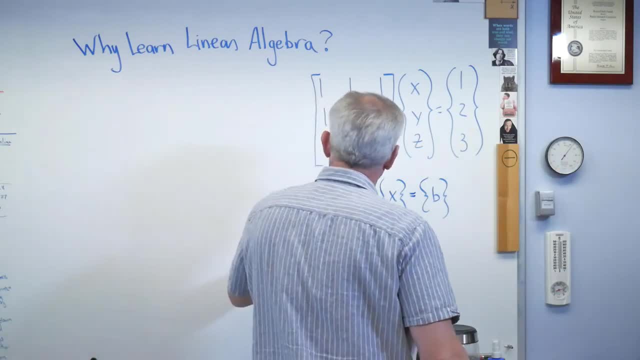 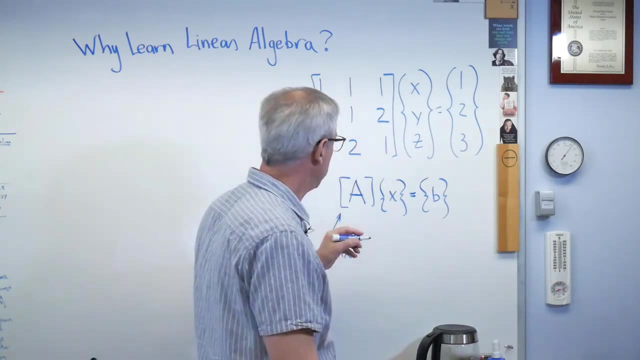 What's a box of numbers called? It's called a matrix, all right. What's a column of numbers, or sometimes a row? That's called a vector? all right, Let's call that a vector. What's that? Well, that's also a column of numbers. 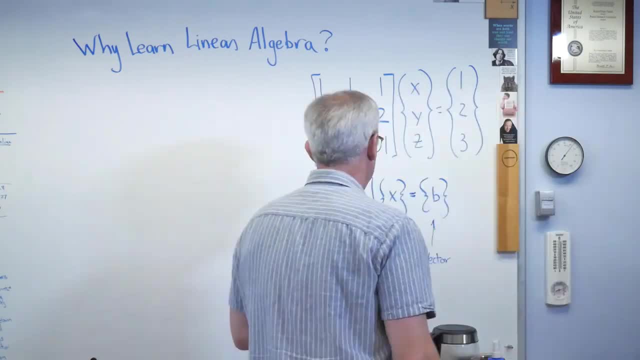 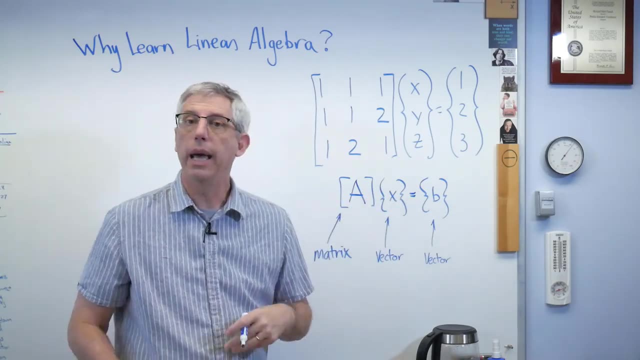 that's also a vector, so we'll just do that. Okay, so now I can work with this a, this x and this b as algebraic entities. and here's the thing, gang. Here's what makes this just so cool. 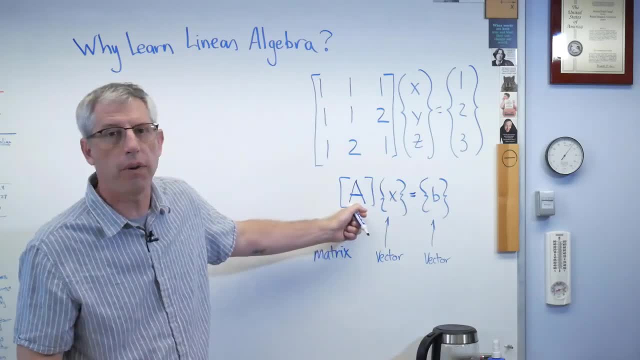 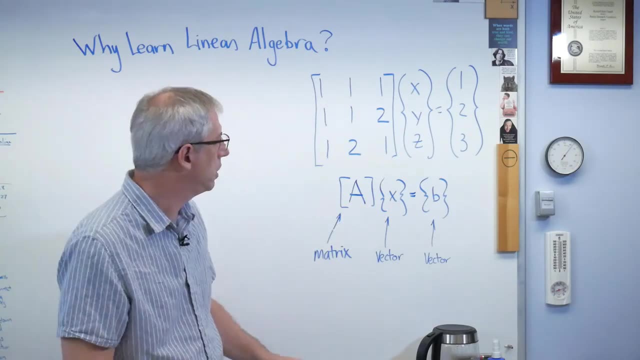 I don't care how big these are anymore. I don't care if a is 3 by 3 or a million by a million. A million by a million, that's 10 to the 12th, That's a trillion numbers. 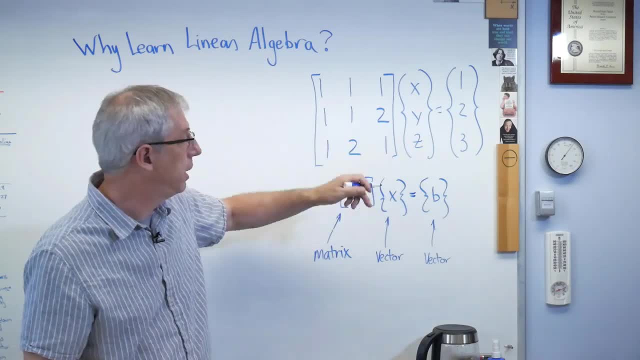 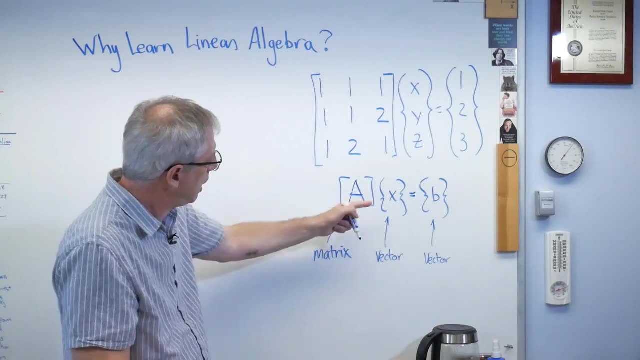 and it acts just the same as if it only had nine numbers. This is a big deal. This is interesting, This is powerful. So how do I solve for x? Okay, now that I've got it written down in this more abstracted form. 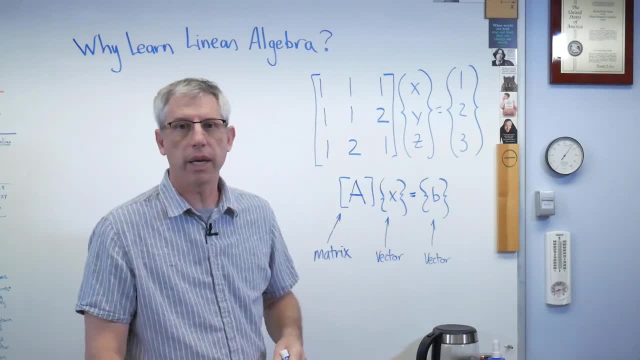 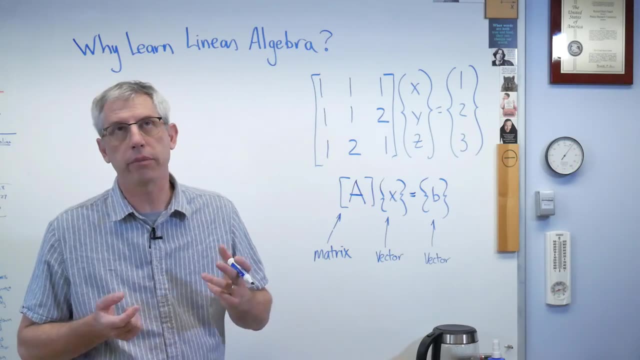 now I can push it around. push these around, just like any other variables. Here's the thing, though: Linear algebra has some slightly different rules than the algebra you may have learned in, I don't know, junior high school probably, but very slightly. 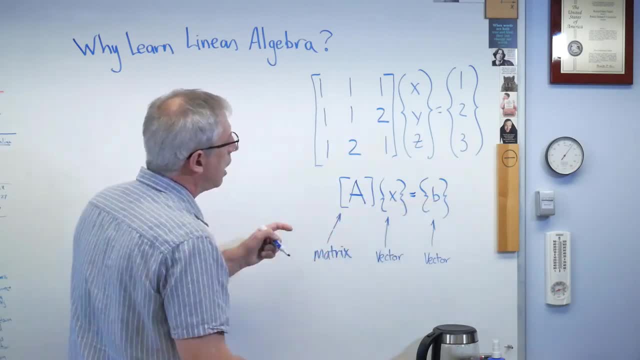 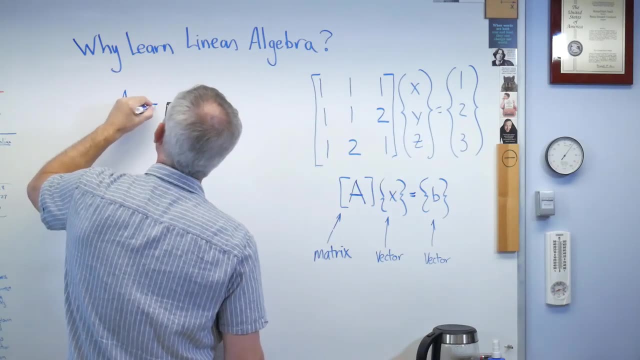 So, if you don't mind, I'm going to not write all the braces and the boxes here, just to keep things tidy. So if I have a system of equations that looks like this- and I want to remind us here, this is a system of equations- 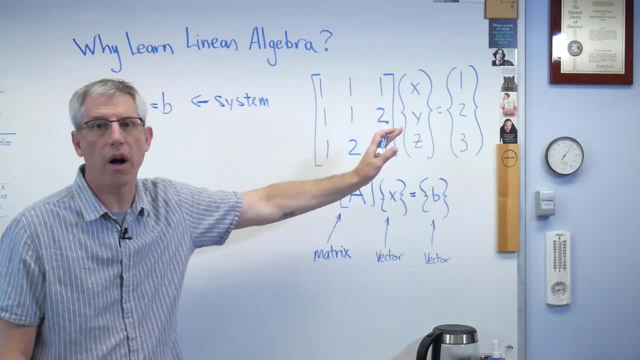 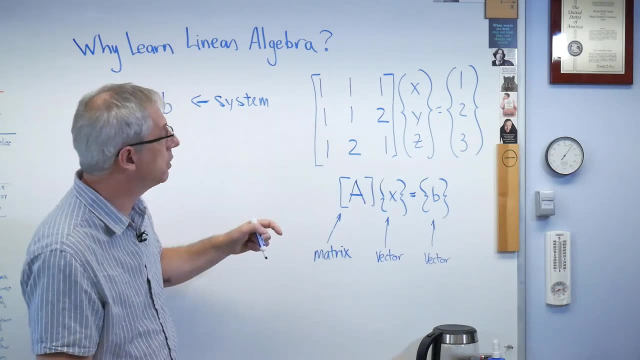 A system means there's a bunch of rows and there's a bunch of columns in this matrix and in this case the number of rows has to equal the number of columns. because of the fundamental theorem of algebra, You have to have as many variables. 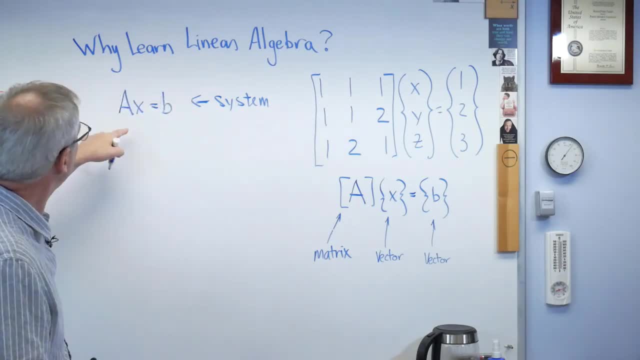 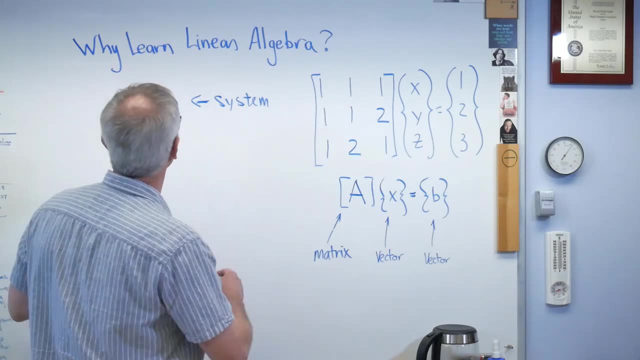 as you have equations, and so that's what we've got. So if I want to know what x is, if these were numbers, x would just be b over a. Well, they're not. These are matrix entities, So, by convention, 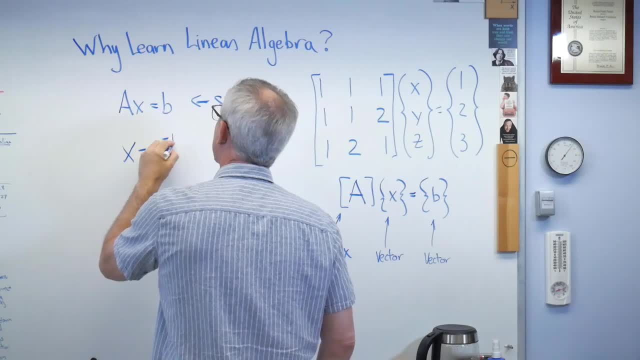 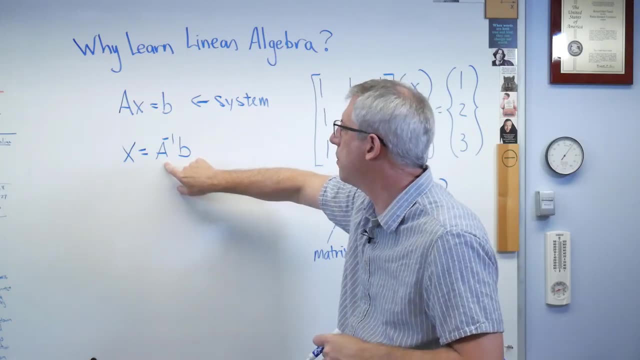 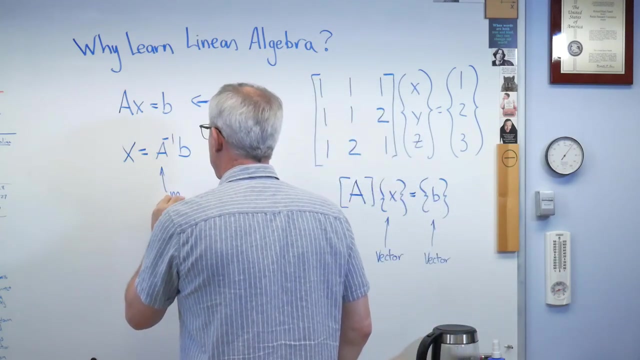 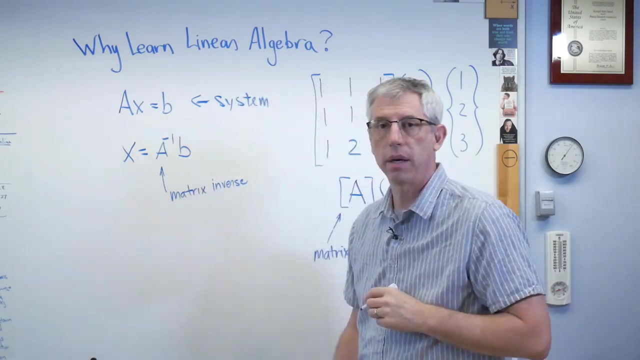 the notation we use. we write it out this way. That's how we solve this, And that a to the minus 1 is essentially 1 over a. I'm essentially dividing b by a. This thing is called a matrix inverse, And there are computer algorithms. 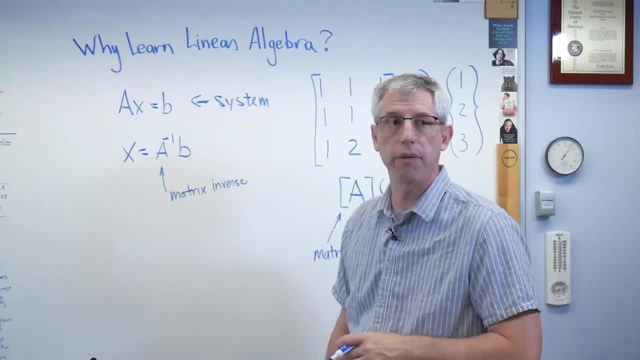 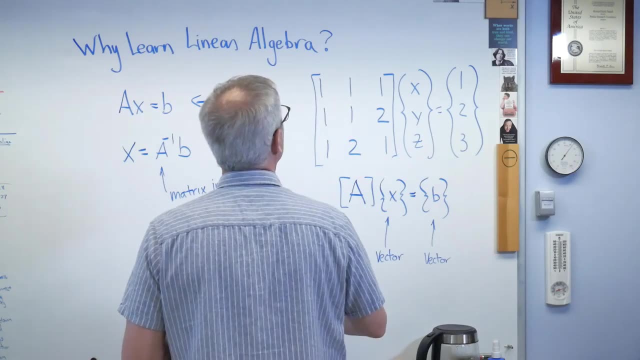 that'll calculate matrix inverses for you, and they run really fast. They're very refined. Most of them are very, very efficient. So it turns out. if I want to know what a inverse is, let's just do this. 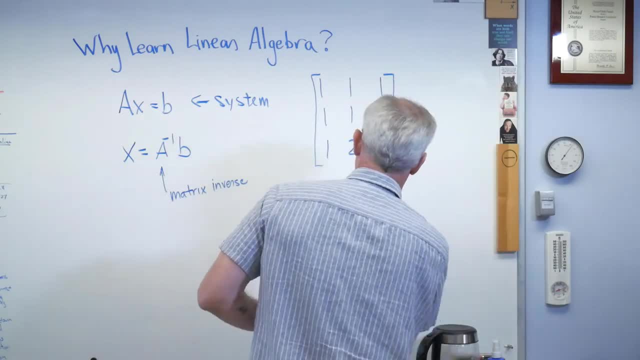 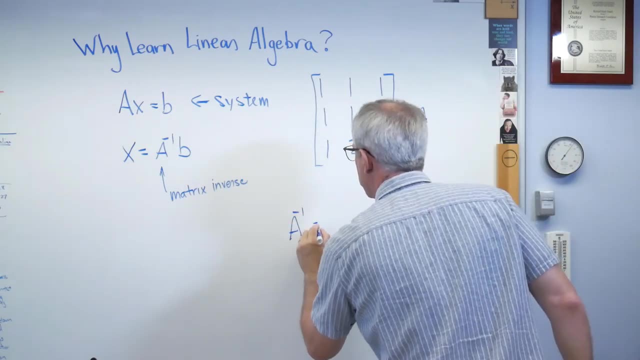 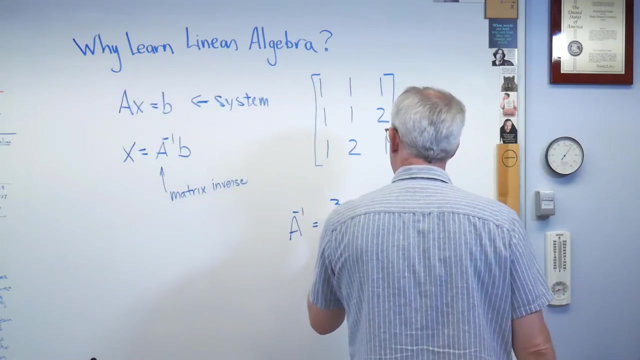 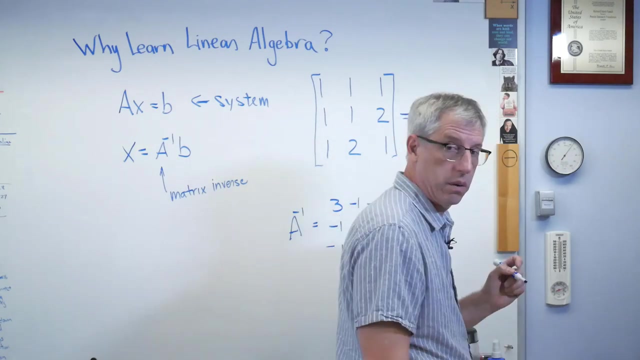 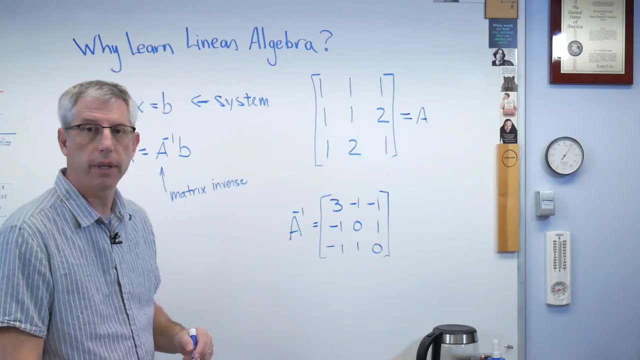 Let's leave that. That's a a inverse. and I did this on the computer. I typed this into a program and I'll write it out here for you. So there you go. There's a inverse, Okay. So how did I get from there to there? 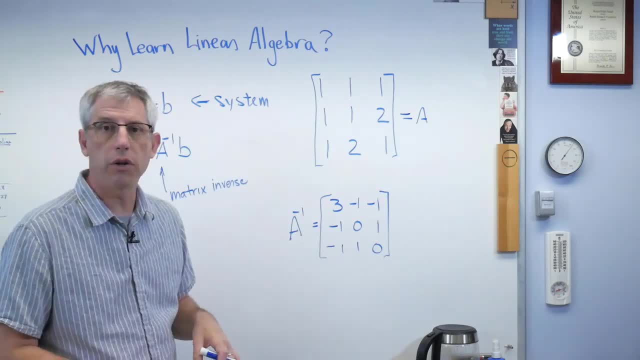 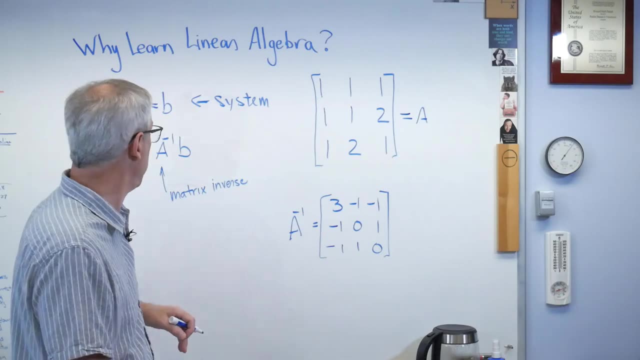 I'll tell you about that in another video. It's not very hard to do. Anybody can learn it For right now. let's not worry about it. It's important later, but right now it's a complication we don't need. 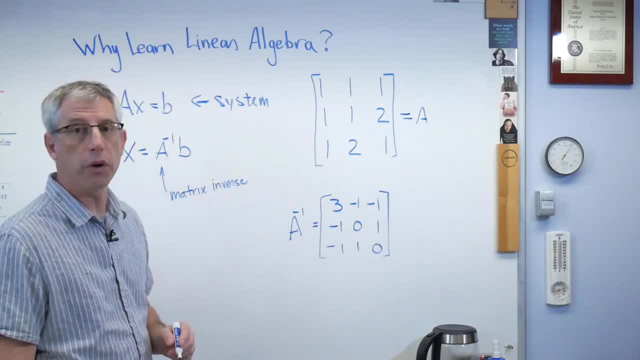 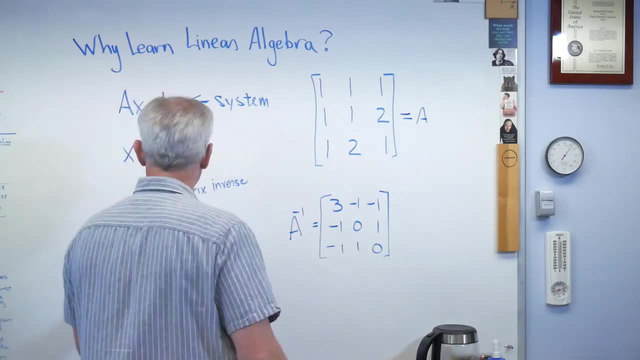 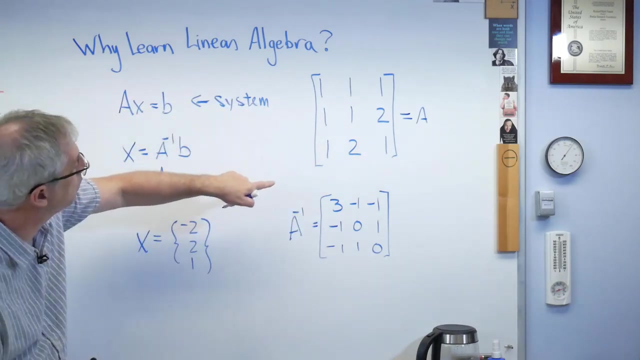 Now I've worked this out on the computer and I'll just write it out for you. In another video I'll talk to you about how to actually make these numbers come out, And that's when I substitute that in for a, to the negative 1,. 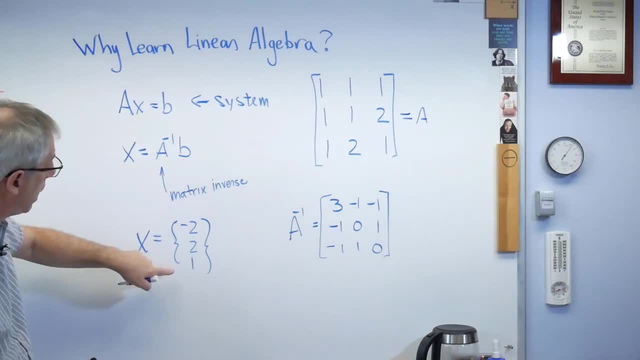 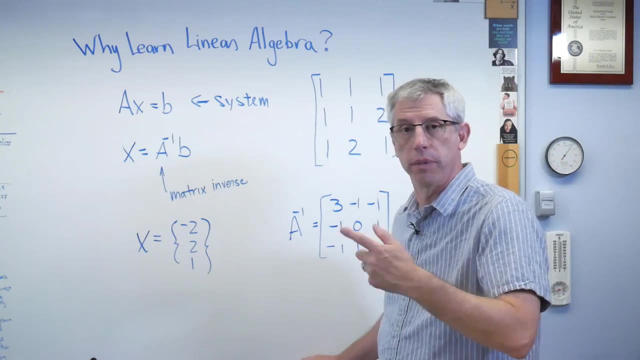 the inverse of a and that b was 1,, 2, 3.. I get that That's the solution. This is the exact same solution you'd get if you went through the whole substitution thing. So that's the mechanics of one simple problem. 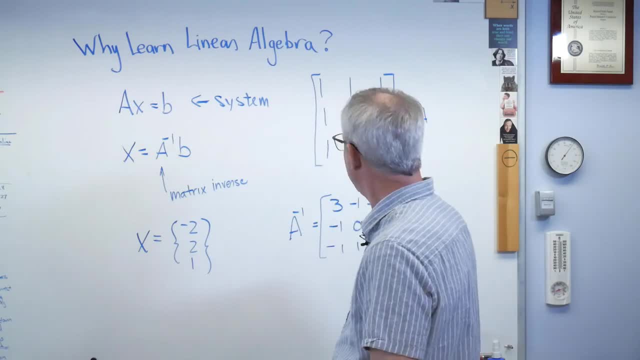 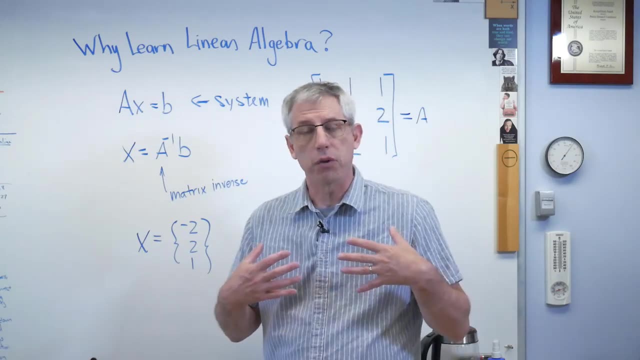 That's how it works, But so far, all I've told you is how it works. I haven't really given you a good reason of why to do this. All right, There's one really big reason, and that's that many, many physical problems. 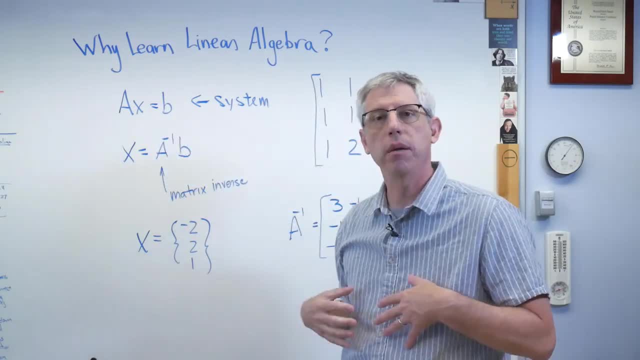 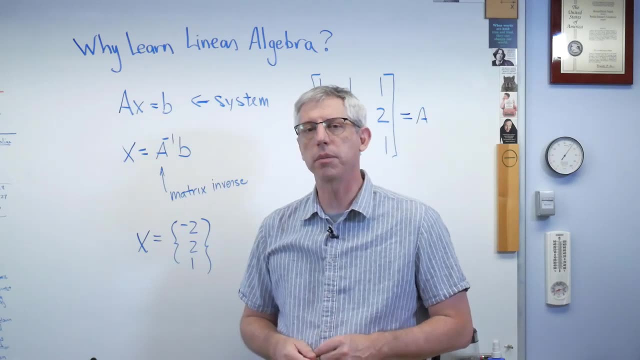 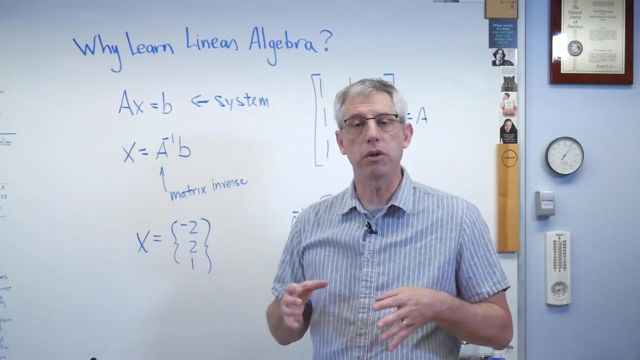 can be written like this. They can be written as a system of linear equations. The world around us isn't that linear, but it's approximately linear. in a lot of cases We can write a system of approximate linear equations and use those to describe the nonlinear world around us. 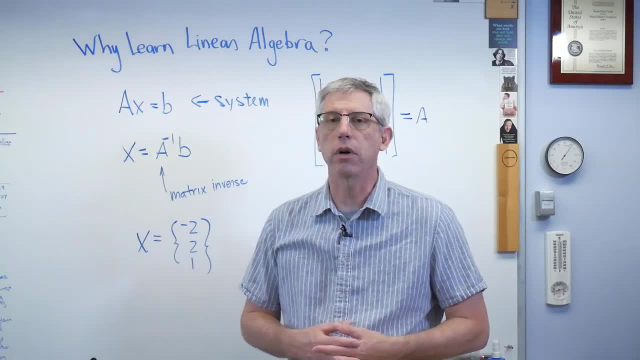 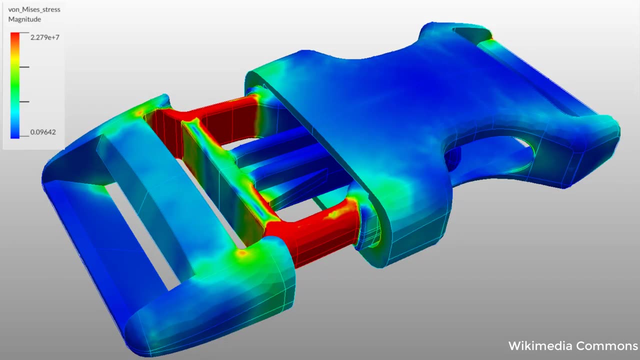 It happens all the time. If you've ever heard of finite element analysis, there are linear and nonlinear finite element analyses. By far most of what gets done in the finite element world is linear. So if you look inside a finite element program, 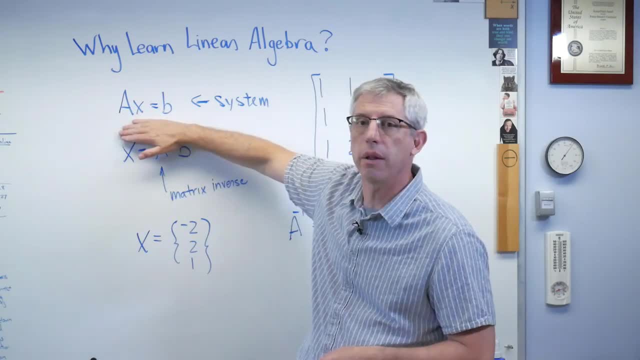 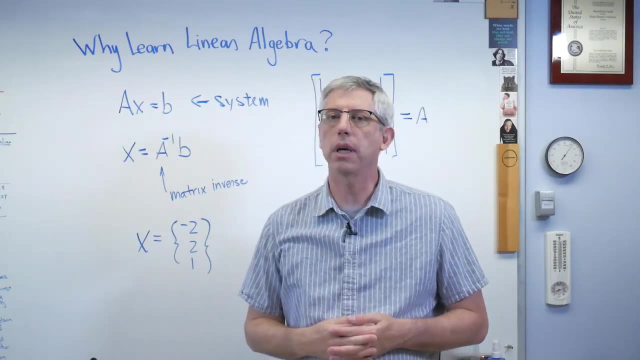 and you know how to look. that's what you see a lot of the time. If you want to calculate displacements and stresses, that's what you're doing. Many, many other physical processes can be linearized about a point. So what you do is you take the nonlinear system around you. 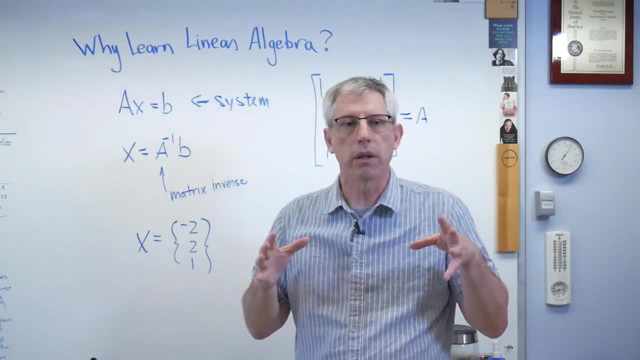 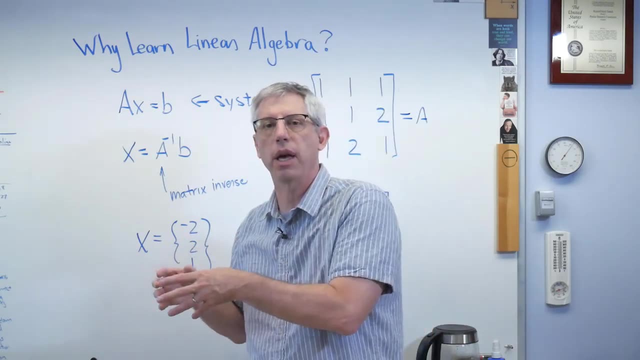 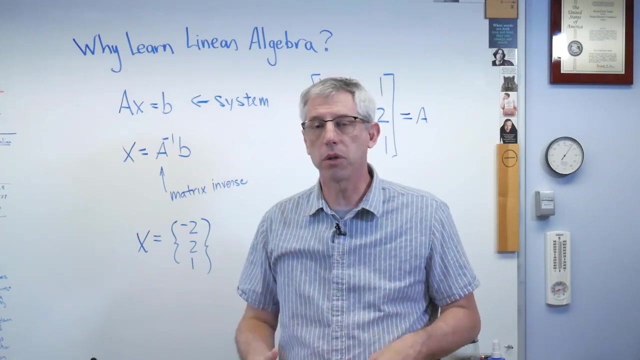 the weather, aerodynamics, whatever. linearize it about a point, solve that step forward in space or time or something. re-linearize, solve again. re-linearize, solve again So many, many, many physical problems in the world around us. 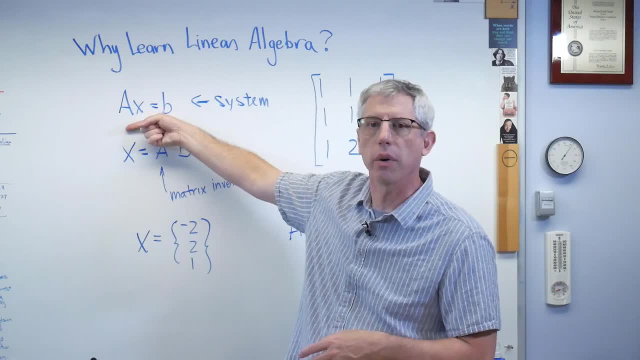 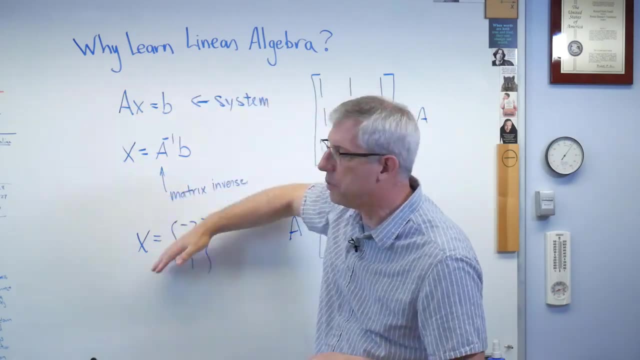 can be written using linear algebra. It's not always this exact equation. There's a thing called an eigenvalue that gets used a lot. There are other linear equations we use, but they still use this basic idea of linear algebra, So one. that's why you want to do it. 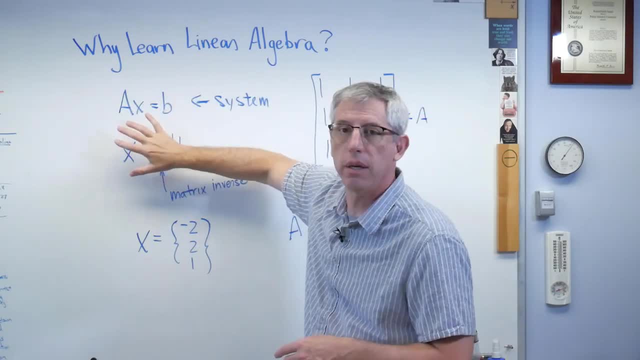 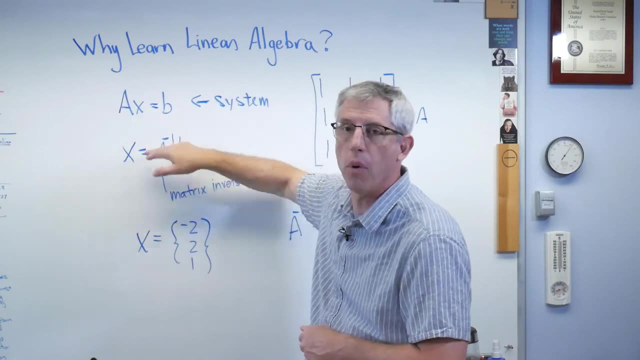 This is being able to work in this now abstract world, this abstracted notation. where that could be three by three, it could be a million by a million. I don't care anymore. That whole back substitution thing just turned into this, That's easy. 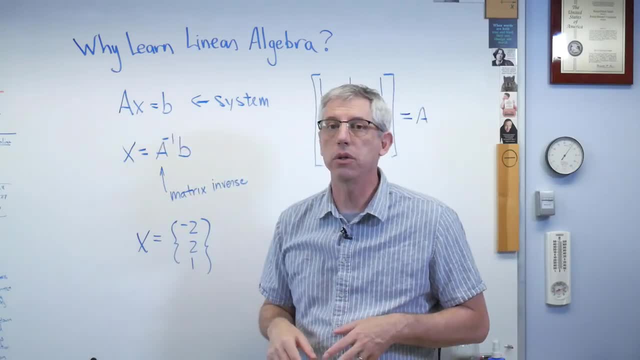 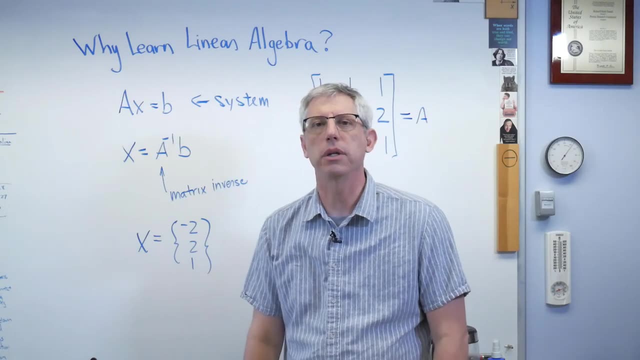 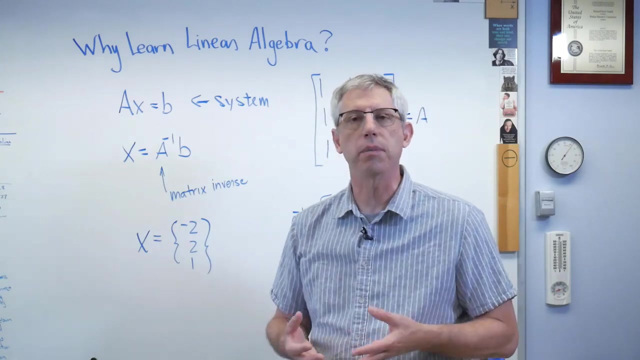 This is very, very useful to calculate the solutions to problems that we find very valuable. So that's why. Now, why is linear algebra such a drag to learn sometimes? Well, the problem- and it is- is because the professors and the students 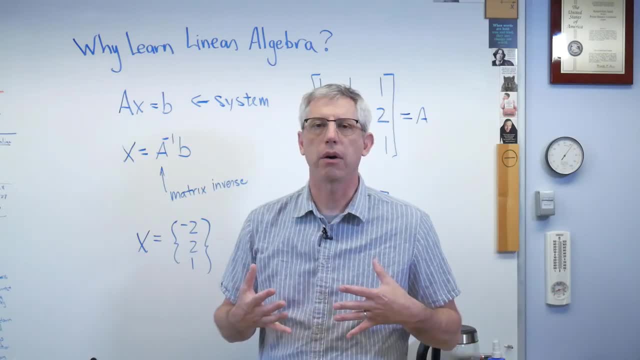 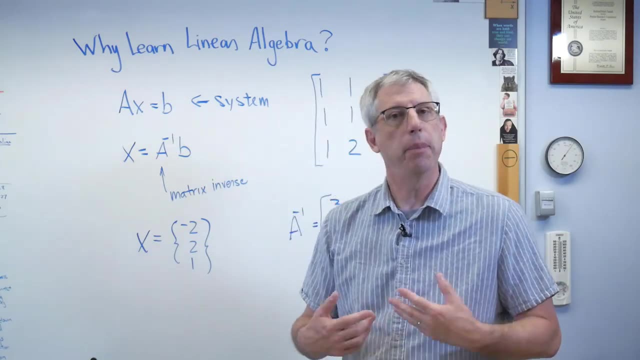 don't think of linear algebra the same way. Neither one is wrong. I want to make this very clear. Both views are completely valid and I think I understand both of them, But as a student, you may not know this, So let me get rid of this. 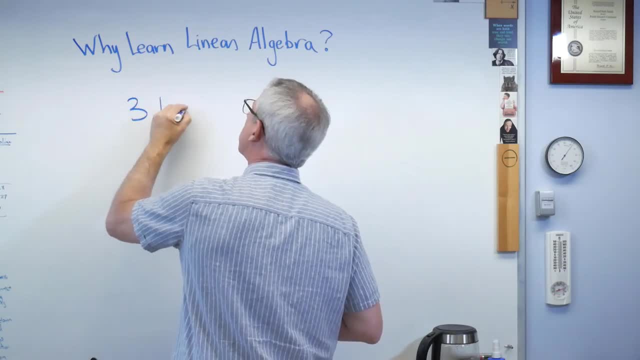 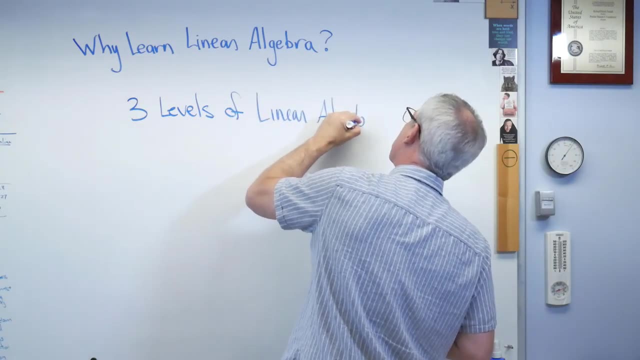 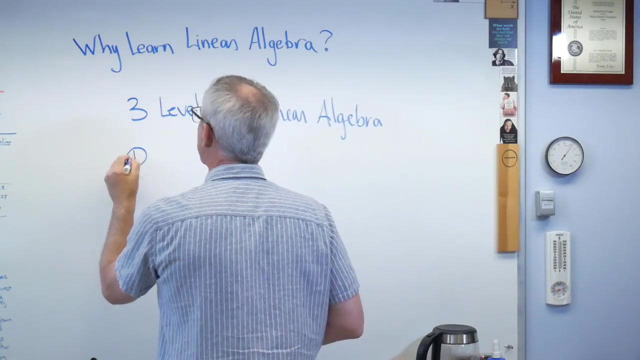 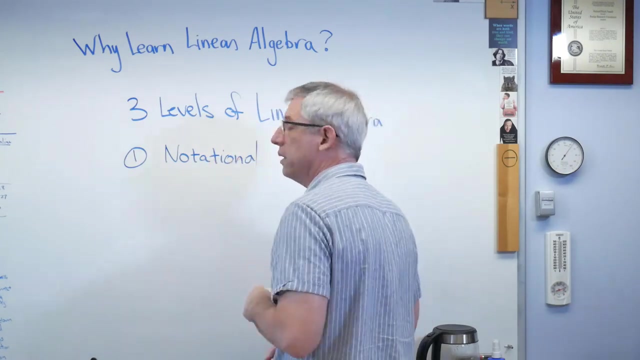 There are three levels for learning linear algebra. The first one is just notational, what we did earlier there. It's just a notation, It's a way of writing out a system of linear equations in a way that's easy to work with. 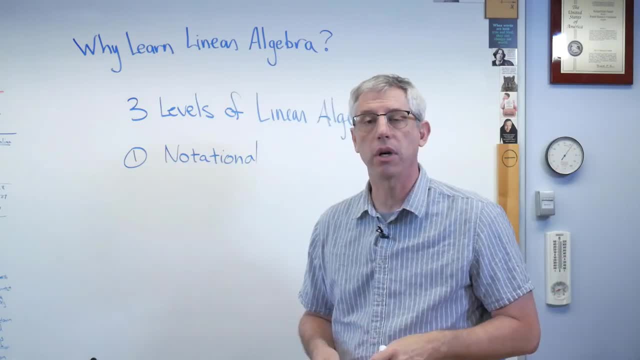 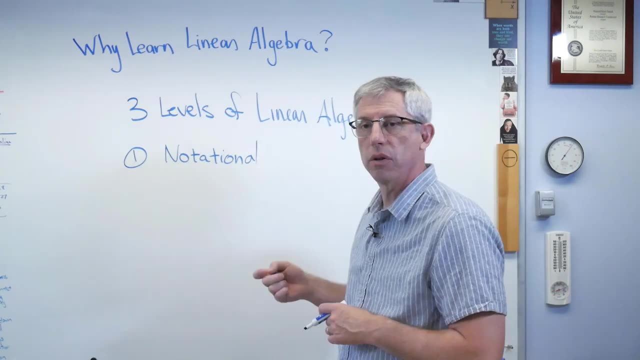 You'll think about it this way if you're trying to type linear algebra problems into a calculator or computer or software or something like this: If you get your TI-84 or whatever it is you've got and you want to solve a little algebra problem, 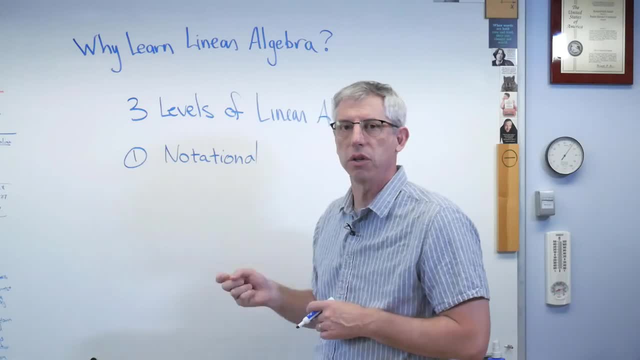 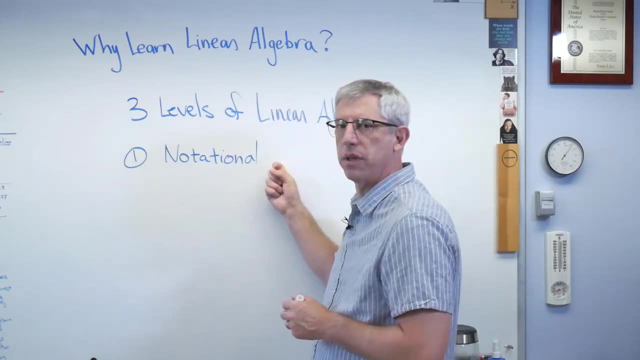 and you want to solve a little linear algebra problem. you can think of it as just notation: What matrix do I type in, What vector do I type in, Hit, solve, and you get your answer. So this is by far the simplest way. 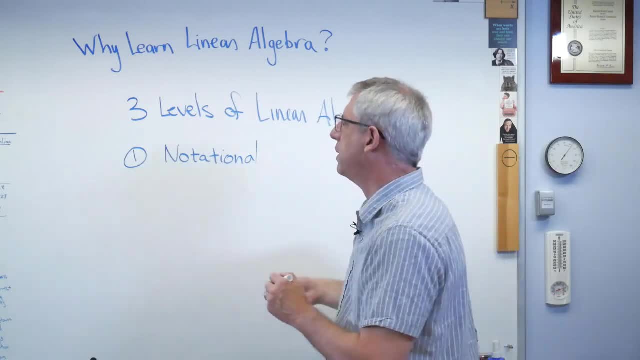 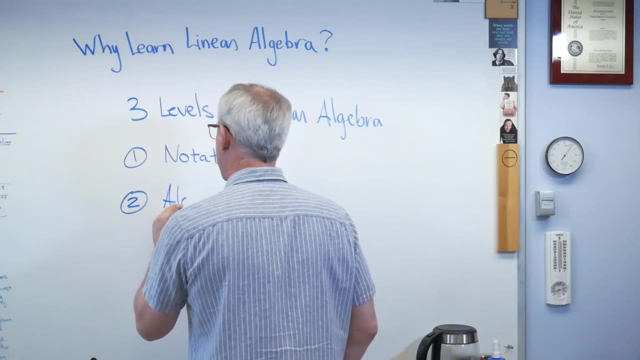 and you probably start here. It's a good place to start. It's not a good place to stop, So the next level is algebra. I don't know really what this is called. I'll call it algebraic. Hopefully mathematicians have a more sophisticated description. 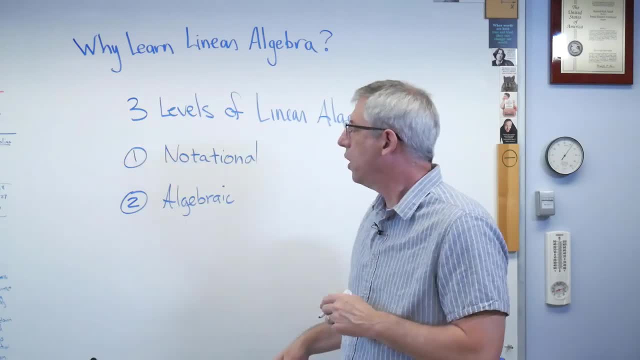 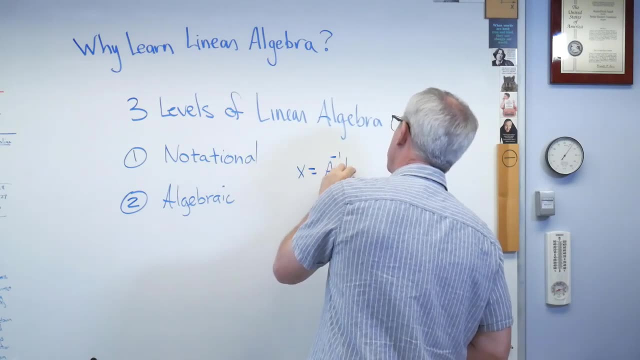 than that, but that's what I got. This is what we were doing over here. When I solve ax equals b and I say x equals a to the minus 1b, that's algebraic. I've gone from the notational idea. 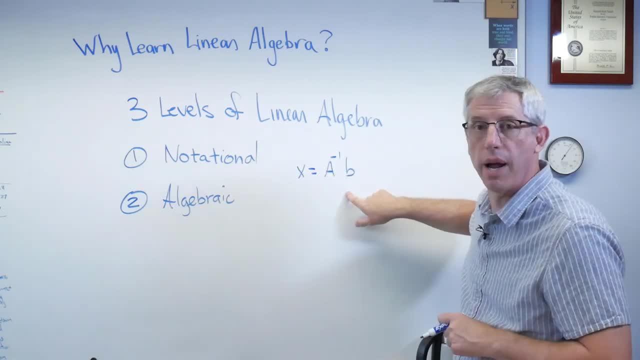 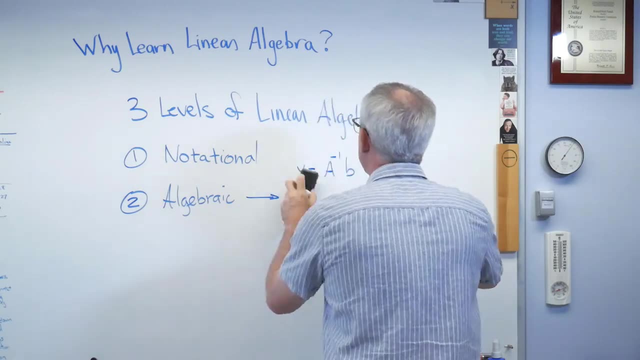 to. I'm actually doing something with it. I'm actually pushing variables around like I would in any other kind of algebra. Well, that's algebraic, and this is where engineers and scientists live- Guys like me. So that's the third level. 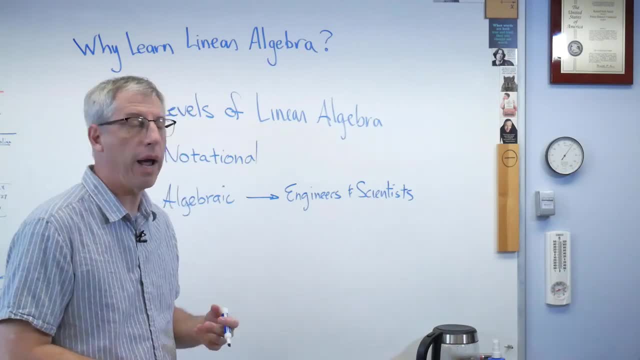 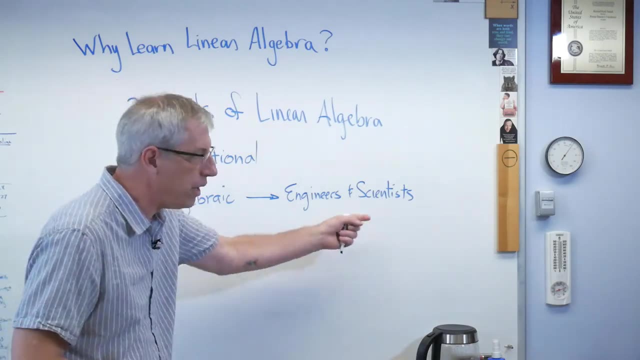 And, like I said, that's where most of us live. When we take a linear algebra class, this is what we need out of it. This is what I got to have If I want to solve a finite element model. I got to know this. 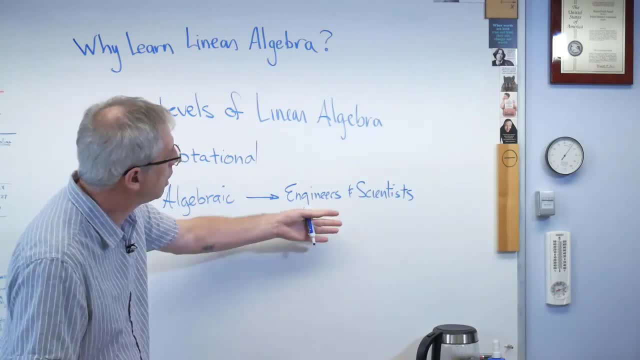 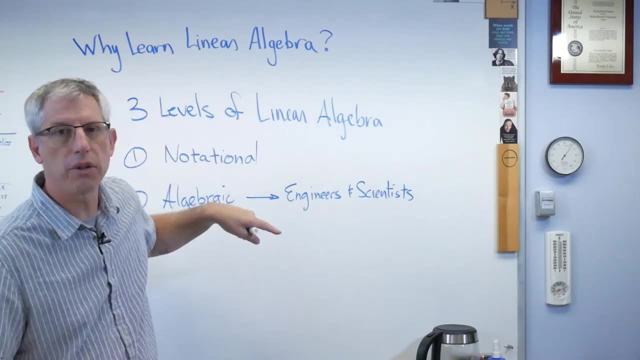 If I want to calculate resonant frequencies of an electromagnetic cavity. I got to know this. This is where the rubber hits the road. This is where this whole notational thing starts doing things for me that I really need. But that's not where mathematicians live. 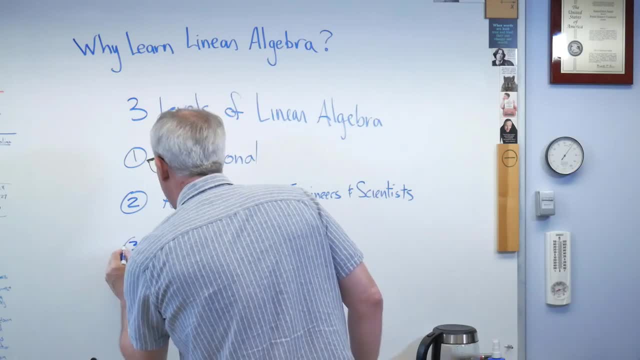 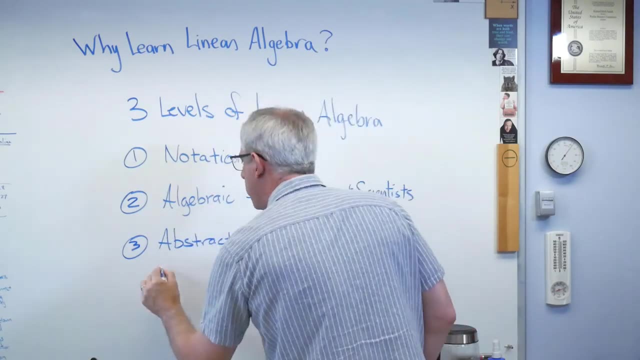 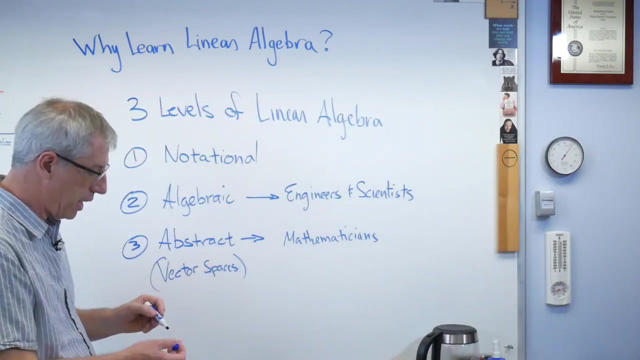 and that's not where they should live. I'm on their side on this one. Okay, What did I call this here? I'm going to call this abstract, Okay. so this is where mathematicians get into it, One of the great advances of mathematics. 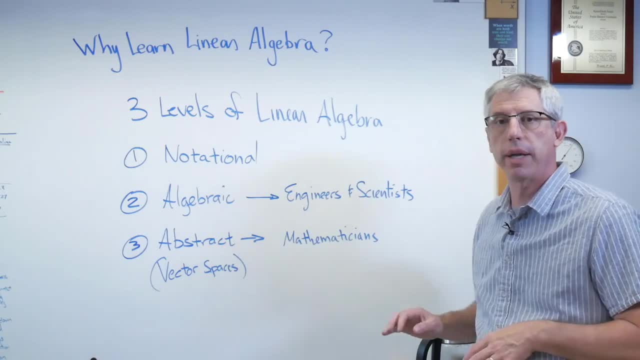 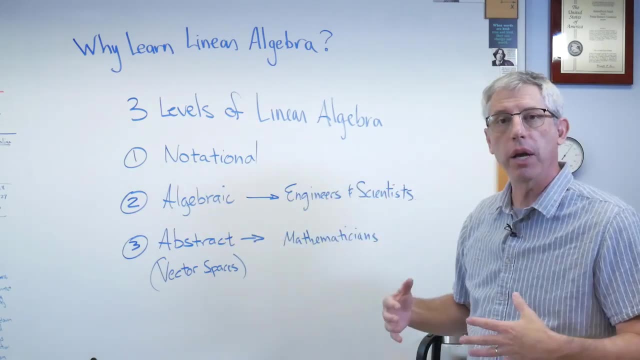 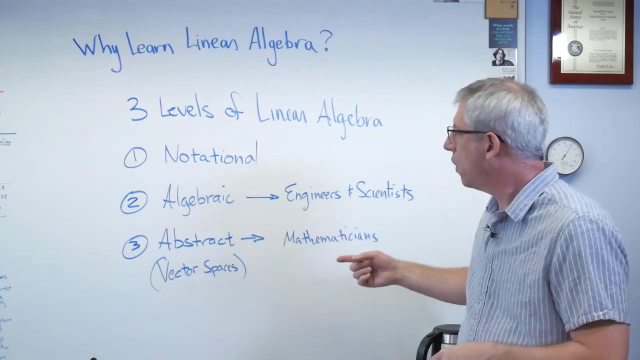 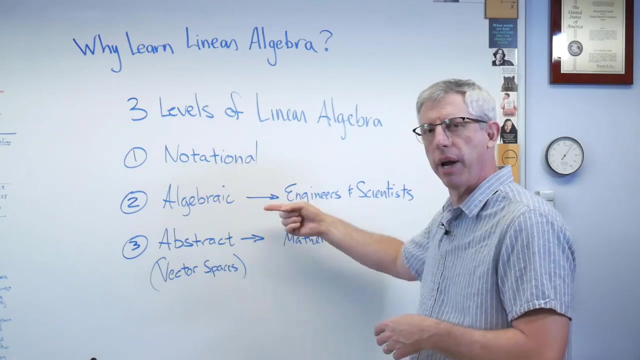 one of the things that makes our view of mathematics now so useful is that the mathematicians are able to start here and start looking for bigger, more powerful ideas that abstract this into something else. So linear algebra developed over thousands of years in algebraic terms. 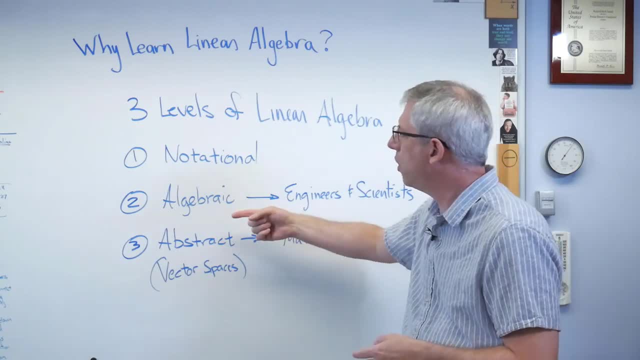 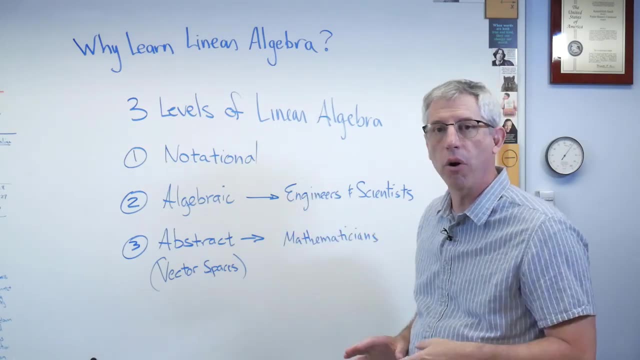 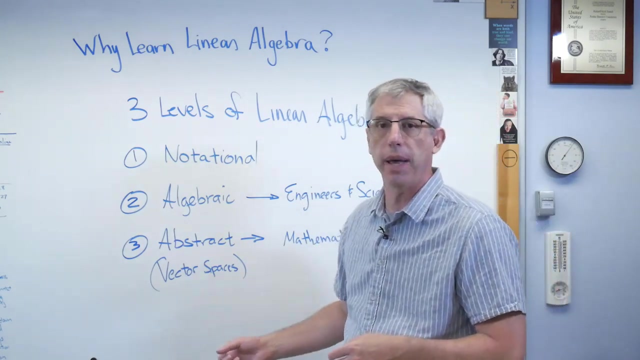 and only later, relatively recently, did people start noticing that these algebraic things we learn to work with obey a more general, a more powerful set of laws, and they're a member of a more general, a more powerful set of ideas, And that's the idea of vector spaces. 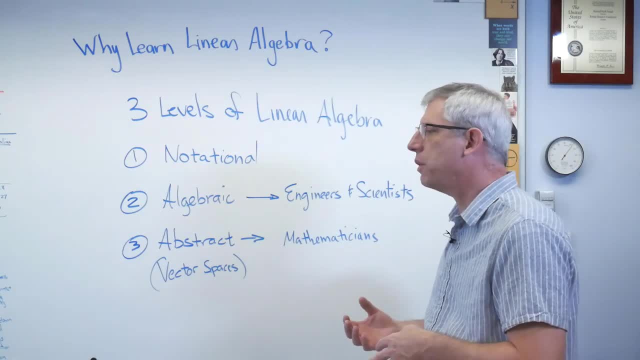 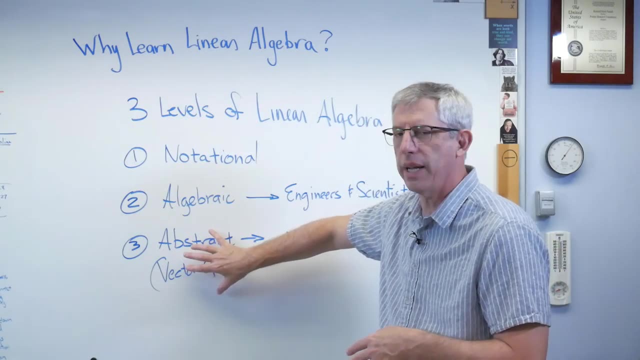 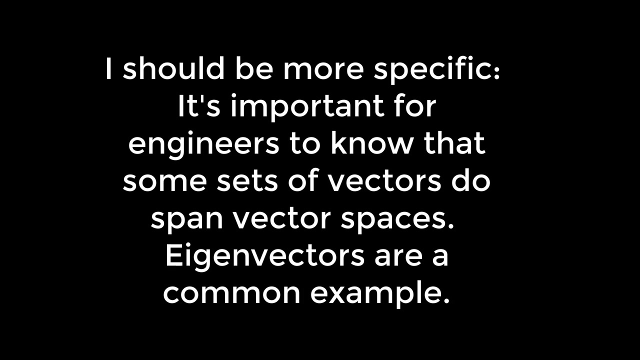 So when you talk to a mathematician they'll wonder things like: well, does a set of vectors span a vector space? To an engineer, there's not a lot of utility there because it's hard to do anything with the result, But to a mathematician, 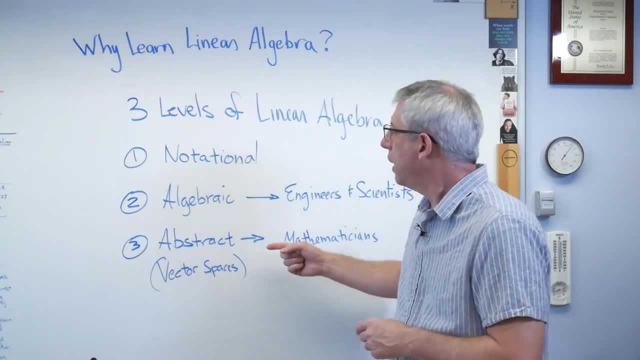 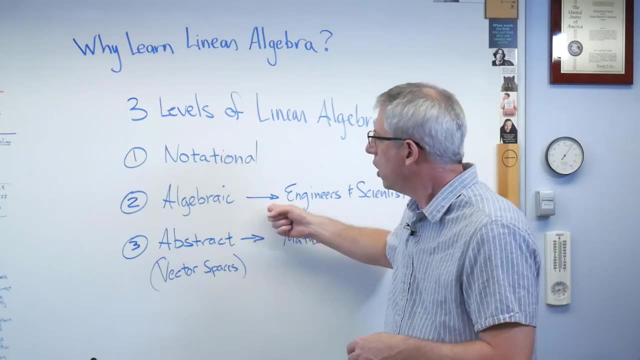 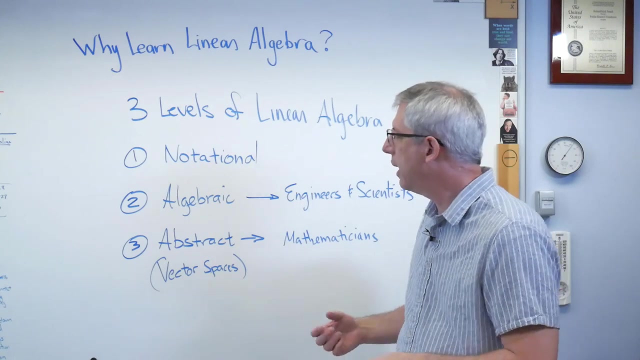 this is exceedingly important and they're right that when you start here, this very workmanlike procedural way of getting answers, you want to find a larger idea, a larger way to think about it, a more general, more abstract way to think about it. 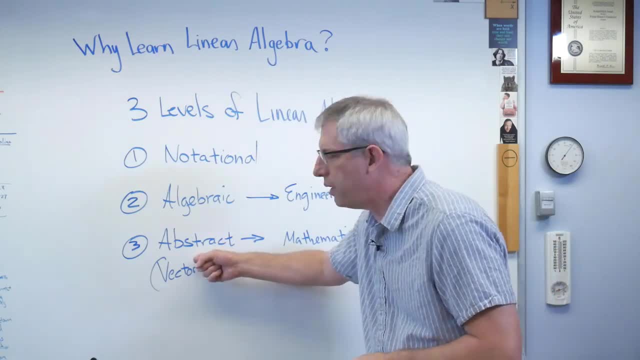 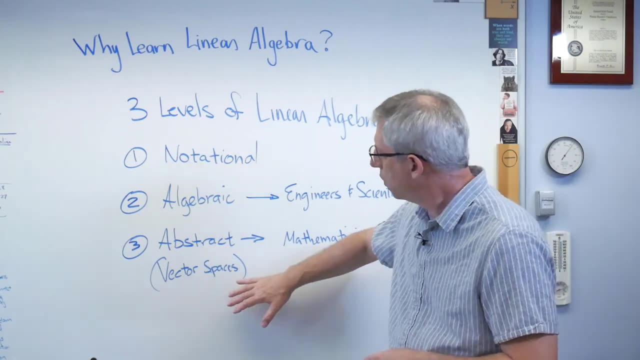 The problem in classes, I think, is that people who think this way are trying to teach people who think that way, And the intersection of those two can get a little rough. So when you hear a teacher talk about vector spaces or set theory or something like that,